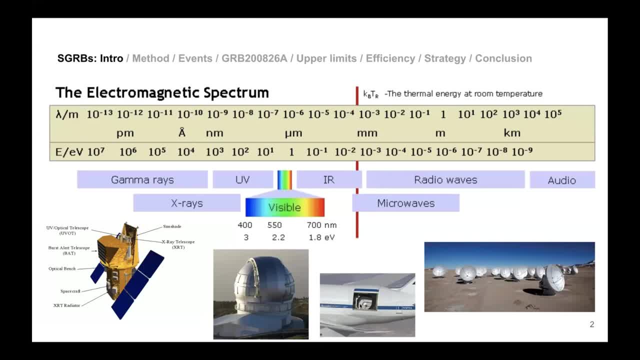 You have to fly out something like a telescope here. This is a plane, It's called SOFIA and SOFIA has a little telescope that is observing in the infrared. And why do you have to fly it? Because our atmosphere is absorbing all the infrared that comes from space. 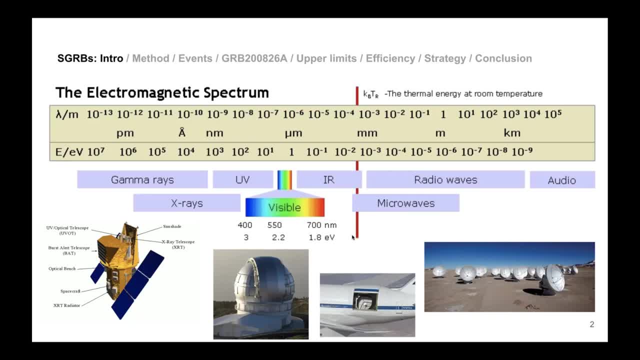 So you also have here a little notation here. So if you are at room temperature you're emitting at infrared wavelengths, And we know, for example, the sun is much brighter, so its blackbody spectrum has its peak in the visible, And visible light can be. 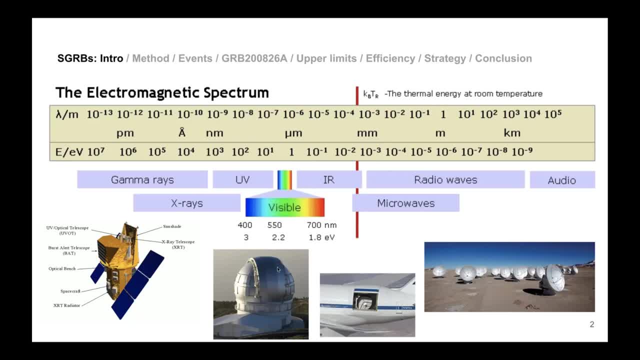 detected with normal telescopes. that you know are much more common. But when you go to higher energies or shorter wavelengths like these ones- gamma rays, X-rays and UV- you have to fly out in space because our atmosphere also absorbs those. So this is the SWIFT satellite. It has a number of instruments like the UV optical telescope. 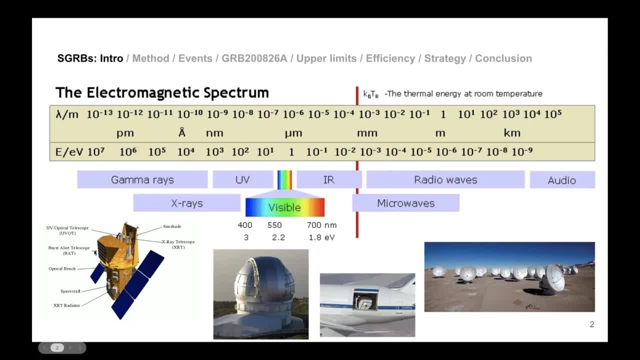 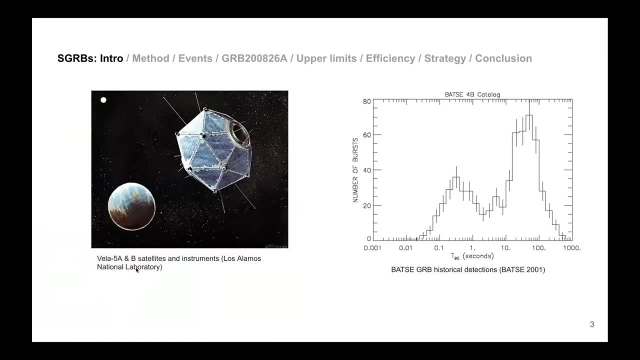 the Bursar layer telescope that it's observing in gamma rays And it's basically a spacecraft that is floating around trying to catch those photons. So I'm going to focus on the high energy part, the gamma ray radiation. How did we discover this? It's very funny because in the context of the Cold War, 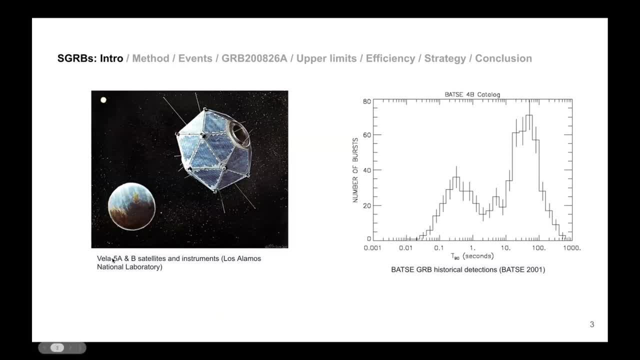 the US launched a few spacecraft called. it was a constellation of satellites called the Vela satellites. They look like this And they were trying to monitor gamma ray activity and they started to find things that were not expected and they did not know where they're. 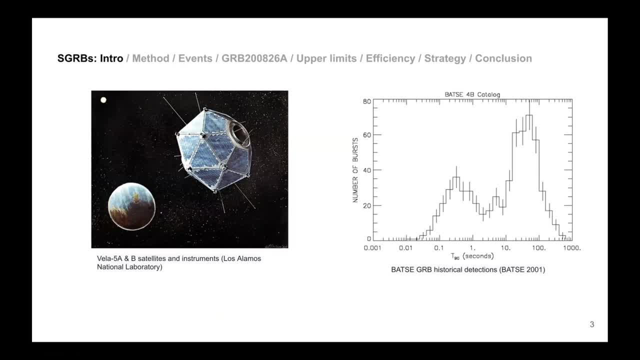 coming from. So eventually, after a long period of time- a couple years- they collected a bunch of them and discovered that they were actually not coming from earth. They were coming from outer space. And they were like: okay, we're not really interested in this, so let the astronomers play it. 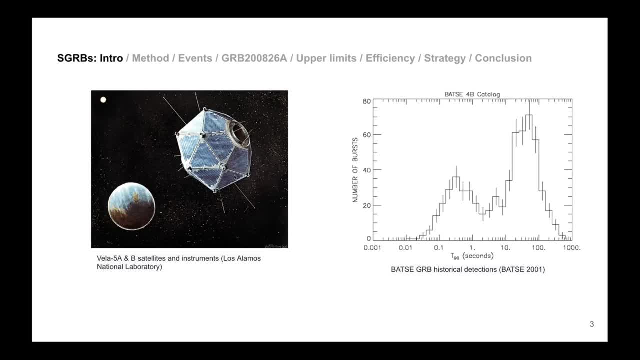 So. So a few years after the BATSE satellite was able to make the first catalog of these gamma ray bursts, So depending on their duration, you can see here a histogram And it basically shows a wide model distribution. What does it mean? 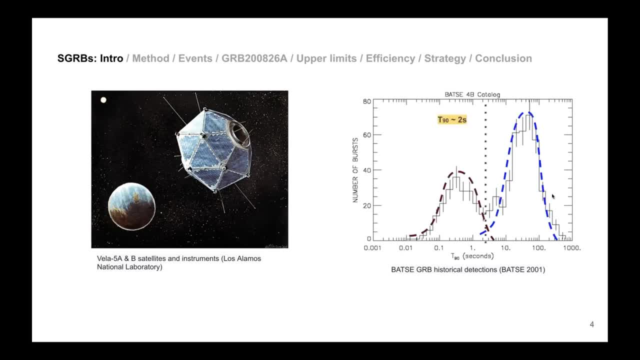 There is a distribution with two peaks, So I'm just showing you basically what are the two peaks You have here, one in close to 0.3 seconds and then another one. this is a logarithmic scale in sort of like 30 seconds. 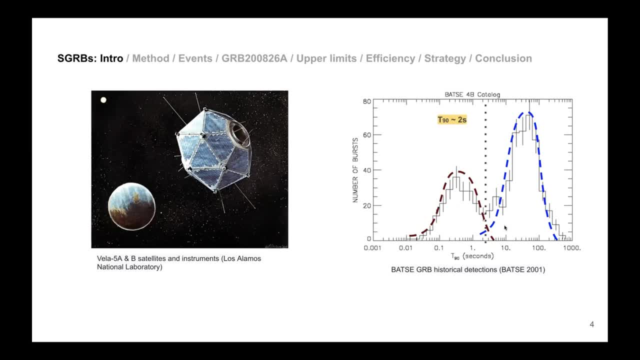 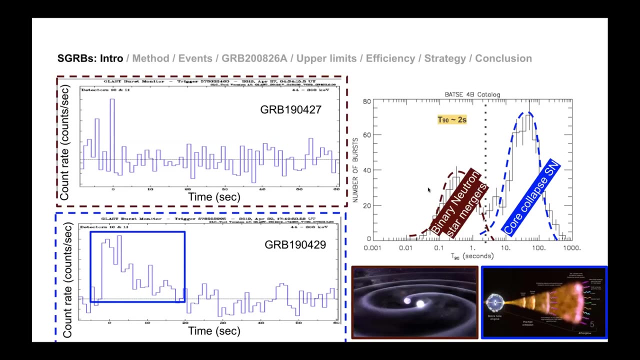 So people at the time were like: OK, if this is true, that means that there are two populations of different sources that are creating those GRPs. So they started studying that with more detail And they proposed that binary neutron star mergers were the ones that produce short GRPs. 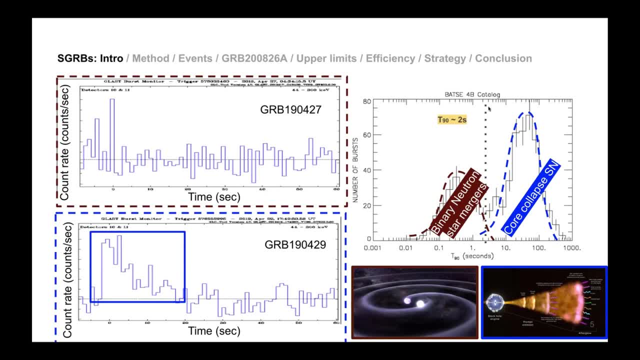 So the GRPs that last less than two seconds. So they put here the division in two seconds And then you have longer GRPs that then were associated with core collapse supernova. So here I have a little picture. These are binary neutron stars. 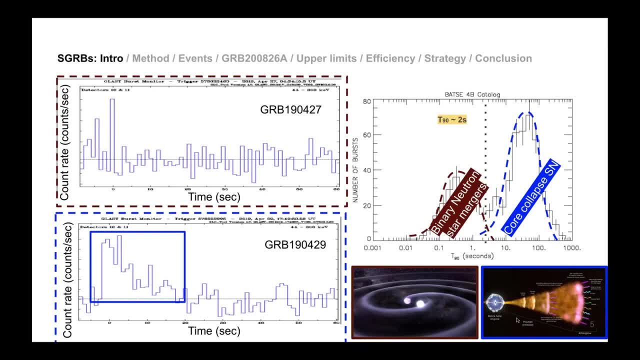 I'm sure that you already know about these, And this is a picture of a core collapsing supernova. I'm here putting and showing you two light curves of GRPs. So what these satellites actually measure is how much photons you get. So you get a count rate. 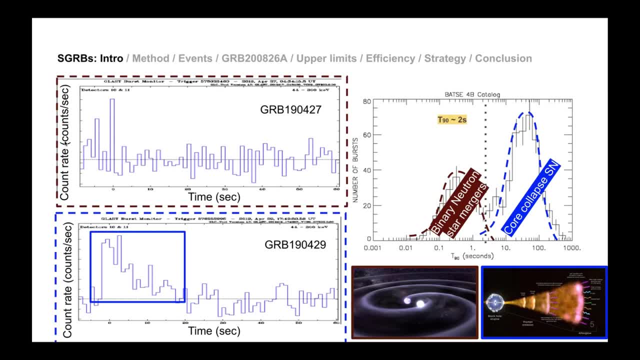 How many electrons are you producing because of the photons you're getting? So for a short GRP, you just have a background, which is this line, And then you have a peak that is less than two seconds. So this is a very bright peak in the gamma ray wavelength. 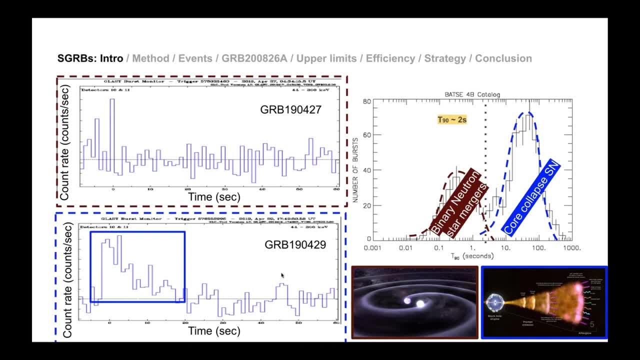 And then you have the energy And in comparison to a long GRP, you have here a much longer emission of whatever object that was collapsing. There is a concept called the T90, which is the duration basically. How did they know that? 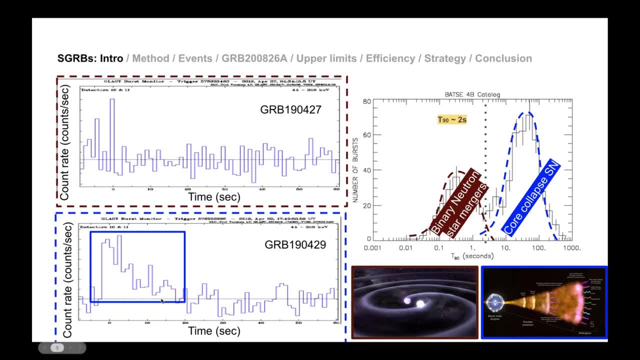 How can we compare the duration? So they actually just take a background level and they calculate what is the duration of the radiation, And then they calculate the energy, And then they calculate the energy, And then they calculate the radiation that is above the background. 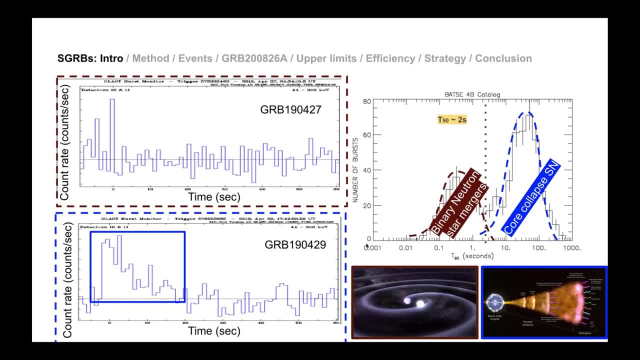 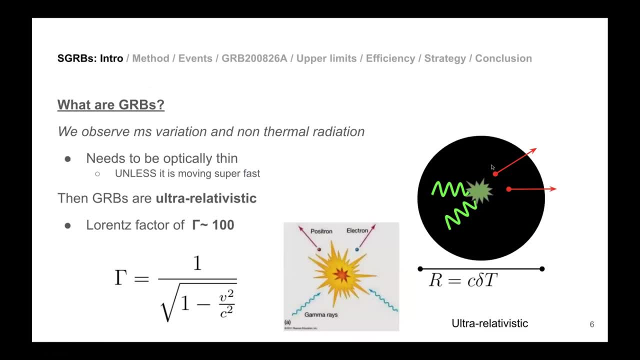 So basically it's just only this part. Then I'm just going to dive a little bit in the history of the GRPs. what are GRPs and what they thought at the time? It was a very obscure thing because you just have a flash of energy that had microsecond variation. 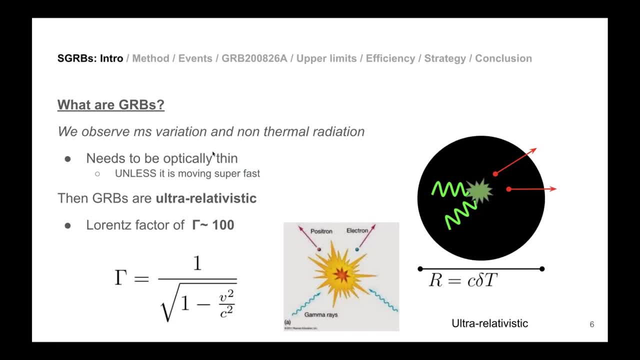 So something that is variating very fast, And you also see that it has non-thermal radiation, So it's not something that is just super hot. So how do you explain that? From the microsecond variation, you can think that whatever is emitting 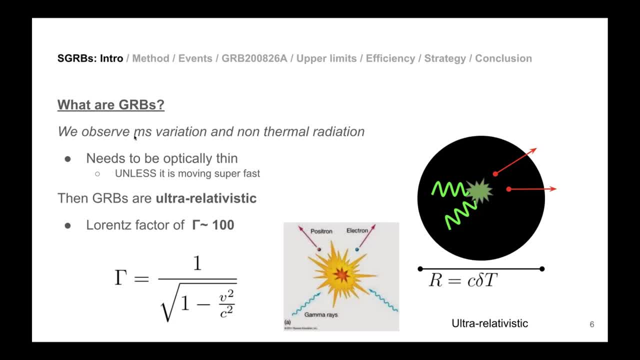 if it's variating on microsecond scale, it means that it's very small. So if you have, for example, this black circle, then I'm not saying there's a black hole, It's just like the region that is variating. 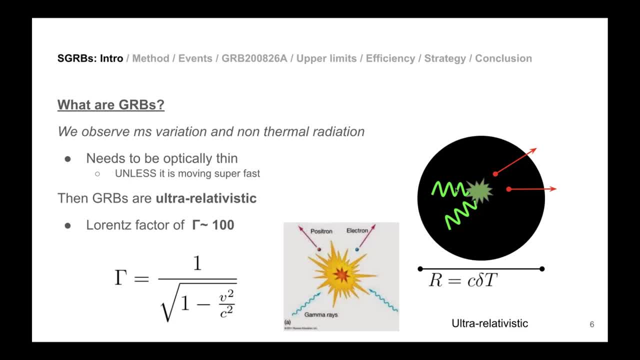 If the information that comes out of the region, the region that comes from this place, travel a few microseconds, that means that the distance that is covering this, it's the other of the few kilometers. So then you need to, since it's traveling that distance. 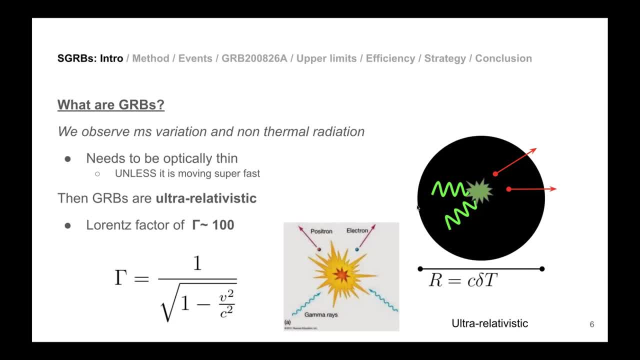 already. you know that it's not being absorbed within this circle here. So there was this problem. because gamma ray radiation can produce, It can undergo pair production, So you have two gamma rays that when they collide they can produce an electron and a positron. 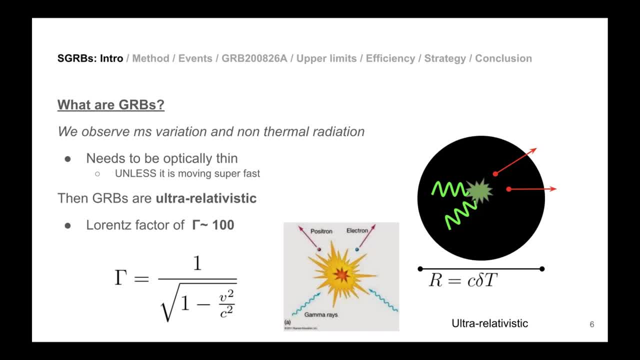 But how can you overcome that if you beam that at a very high velocity? So then the frequencies are double shifted And then it's no longer optically thick. So how do you make this transparent? Well, make it super fast. So then you have here as a conclusion: 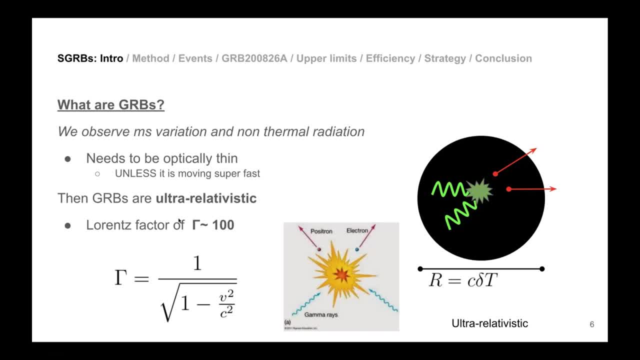 that these GRVs are ultra relativistic. That means that it's going very fast. You have this Lorentz factor that you'll probably keep hearing if you continue in transient astronomy, because there are just things that are exploding, And explosions means a lot of velocity, something. 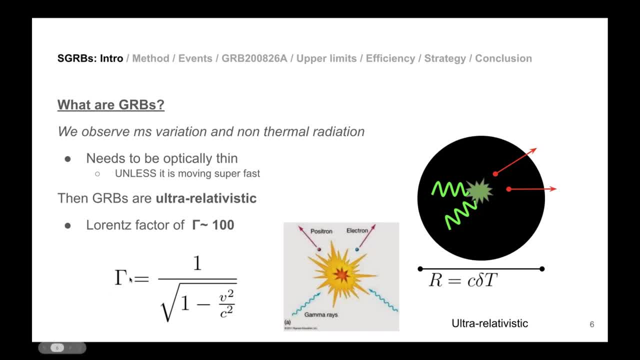 that is very, very rapid. So then you have the Lorentz factor of order of 100, so that the Doppler shift can also a lot of the energy- And I'm sorry, I'm sorry- allow it to radiate outside of the region that's emitting. 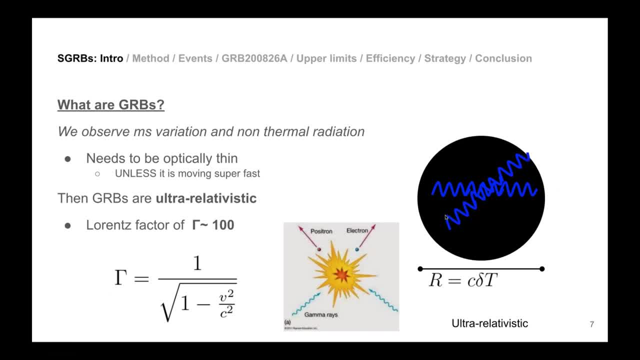 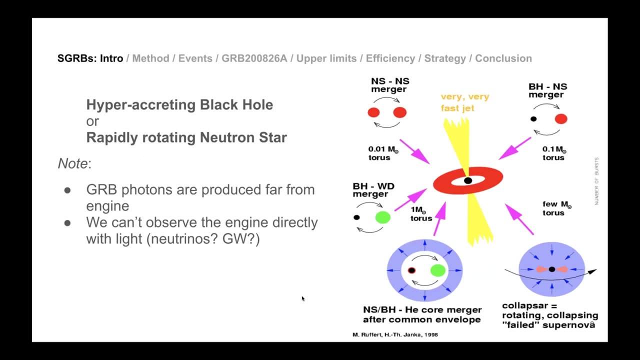 So if it's Doppler shifted, then you have more energetic wavelengths and then these are transparent and they can get out of the region. So okay, so we know that there is something that is very, very fast, very, very fast moving. 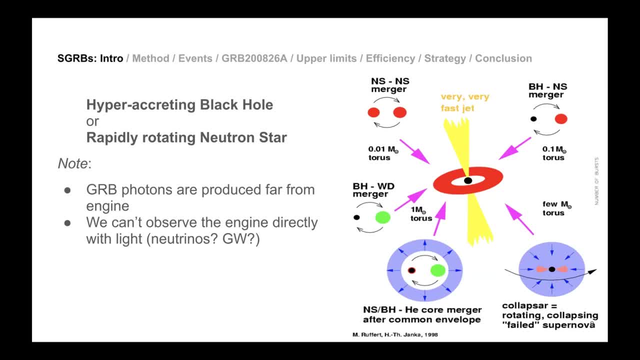 So how do you create those things? That's the main questions. What are the progenitors of those gamma ray bursts? So we know what we can characterize, what we observe, but it's harder to infer what is behind it because basically we have a couple photons. 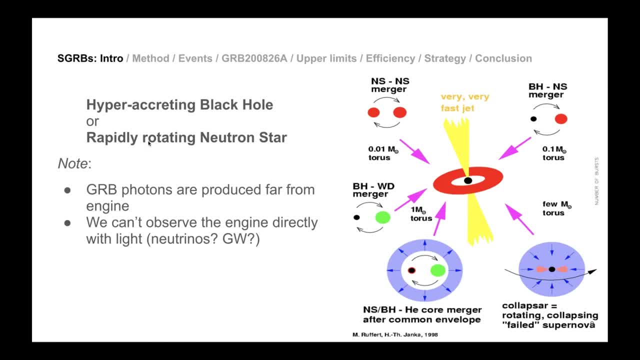 and then we are trying to figure out what is happening with those. So theoretically you have you need to think about basically two things to happen. You need a very compact object that has an accruing disc. So it's either a hyperaccurating black hole. 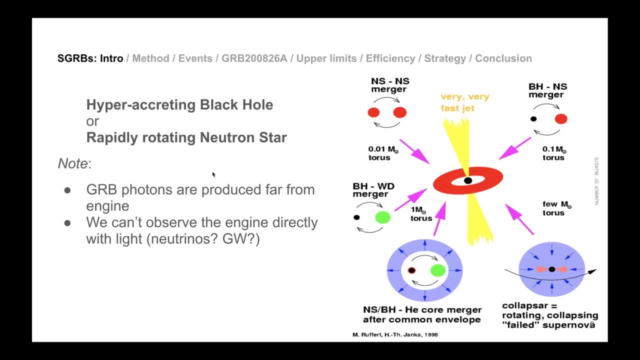 or a rapid rotating neutron star that generates also an accruing disc. So then you have a number of candidates. So you have the neutron-neutron mergers or binary neutron star mergers. here, Yeah, the black hole neutron star mergers, black hole white dwarf mergers and lately the neutron. 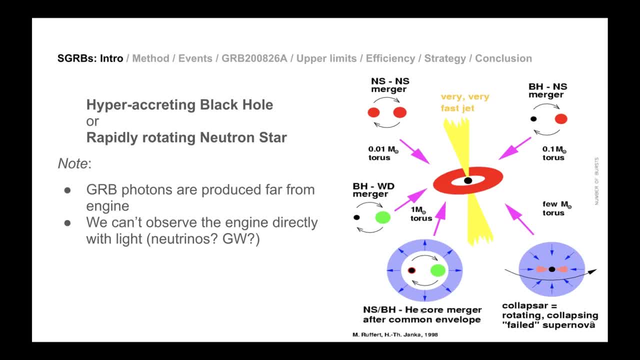 star, black hole with a helium core that merge within a common envelope. So all these have been thought to produce short GRVs. but then you have a collapsing massive star that can also produce those jets, And that scenario is called collapsers. But since these are massive, the scales are much larger. 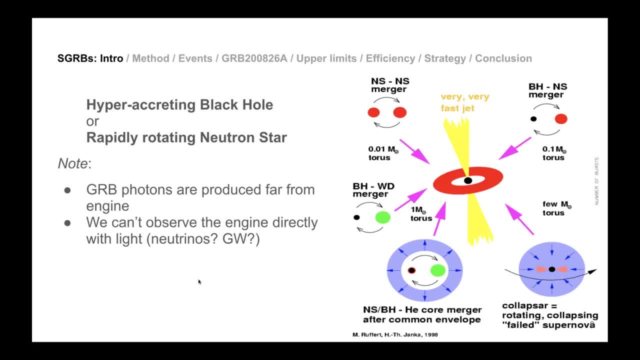 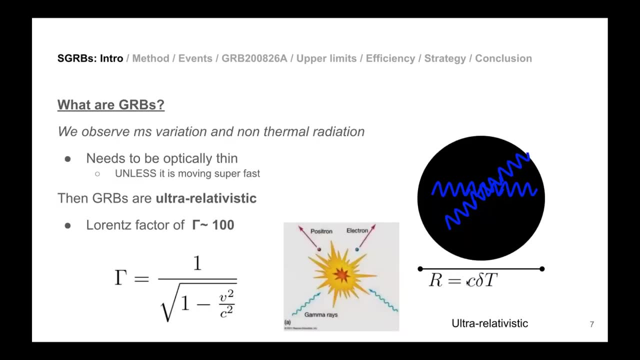 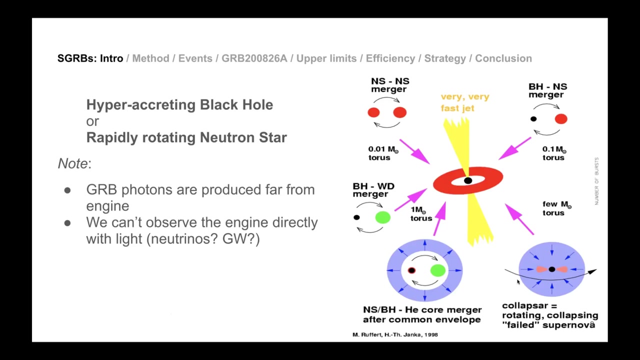 So that's where we think long GRVs come from. Please note that those GRV photons are produced far from the engine. So if you remember that just little hand wavy calculation we did, if the radius was, you know the velocity of the light, times a few microseconds. that gives you a few thousand kilometers. 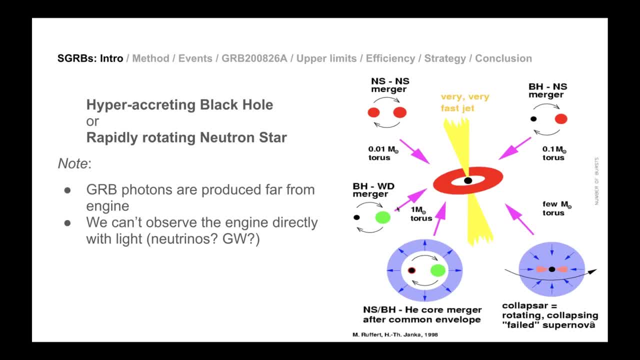 which is basically a little bit larger than what you would expect, for example for a neutron star. So a neutron star diameter is like about 10 kilometers and this is three orders of magnitude. So the gamma ray emission does not occur from the engine, so it's like in the outskirts. 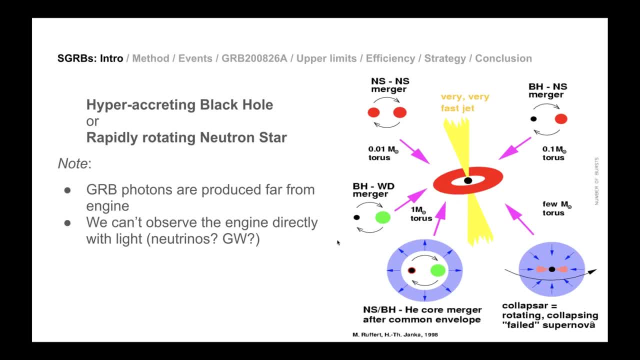 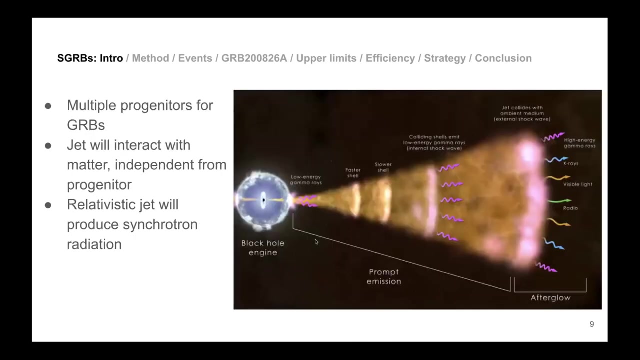 of the engine, Then we cannot observe directly the engine. So you'll probably hear more about how can we get more information about the actual engine from neutrinos later, and you have already heard about gravitational waves, So this is how we can probe the inner part of these explosions. 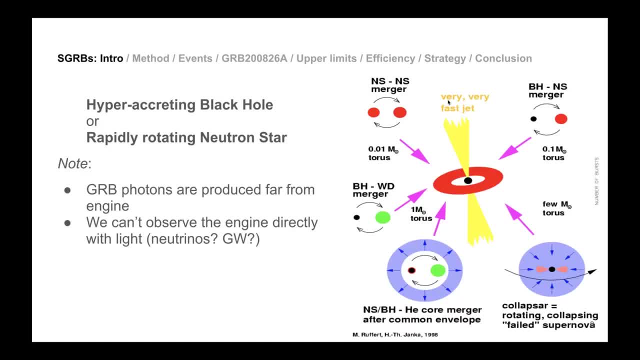 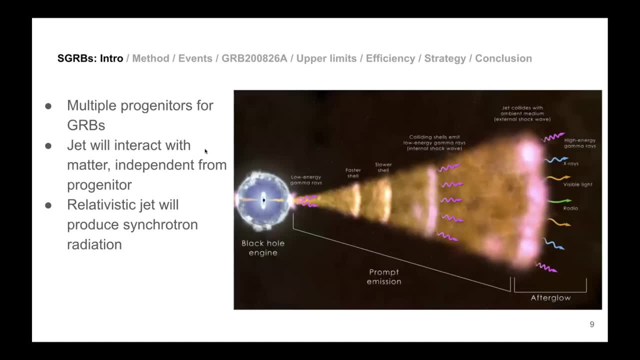 So, as I showed you here, you have multiple kinds of progenitors that can produce short GRV. But once the GRV is produced, once the jet is produced, it will interact with the matter that is outside. We call that circumversed environment. 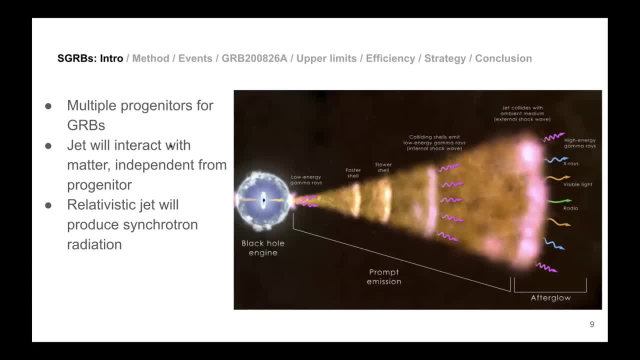 So that interaction it's independent of the projector. So you have here a cartoon model of a long GRV produced by a collapsing massive star. So this is the star. in the center You have a black hole. This is a creating mass. 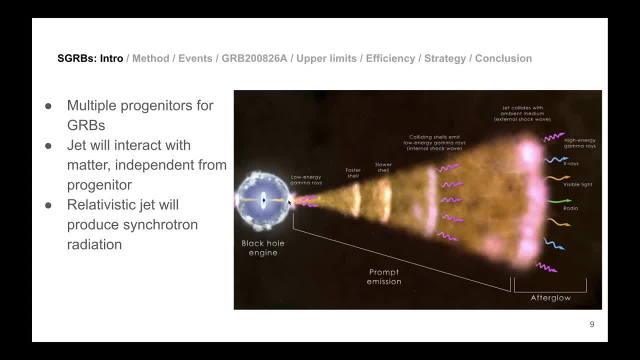 And it produces a jet that breaks the envelope of the star, and then it goes and goes and goes out, And then you can see that, depending on how far it is, how fast it is, it will produce radiation that is non-thermal, that we call synchrotron radiation. 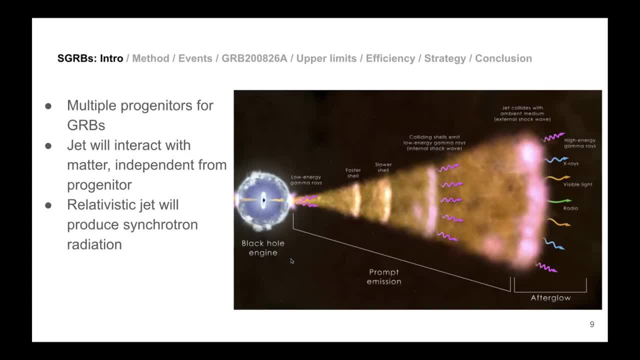 So synchrotron, it's basically relativistic cyclotron. So it's the interaction, Okay, And then you can see that it's moving in the direction of charge particles with electromagnetic fields. So since these particles are moving very fast when they interact with the electromagnetic 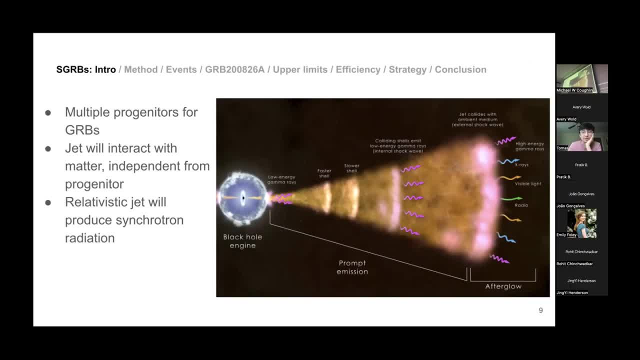 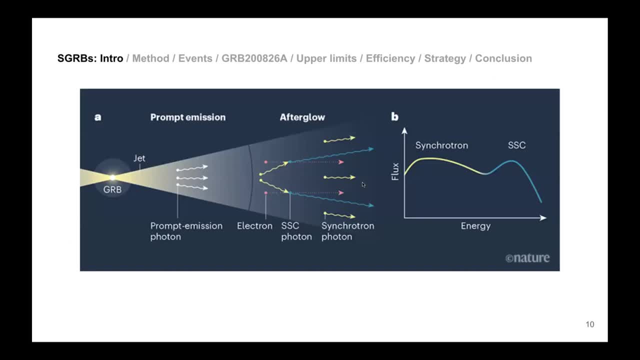 fields, they produce radiation across the entire spectrum. Then you have here: how would it look from Earth? So you have here the GRV. It depends. It depends on what is the progenitor. You have the jet that we call prompt emission. 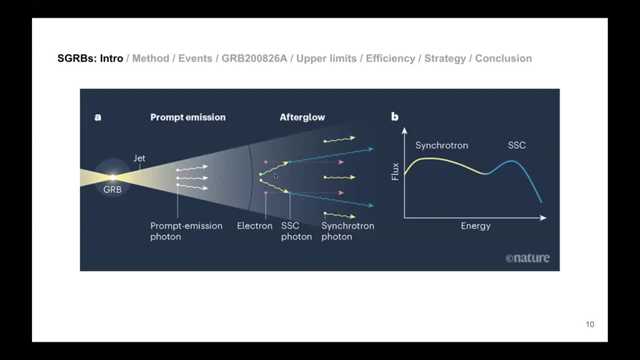 That's the actual gamma-ray radiation. And then you have the afterglow. So this is what happens after You have electrons interacting with light, but also electron interactions with themselves and producing self-compton scattering. So you have here a synchrotron light- sorry spectrum. 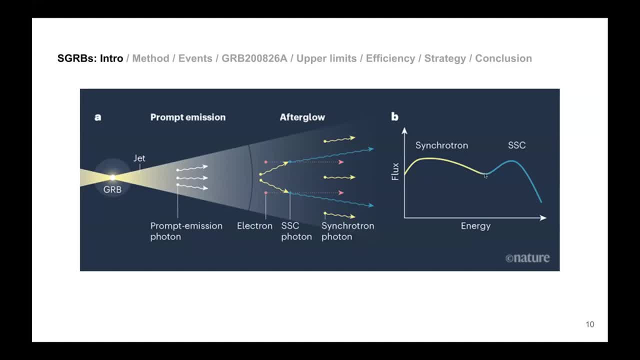 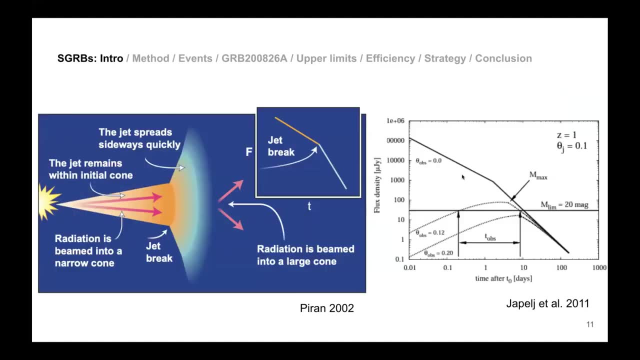 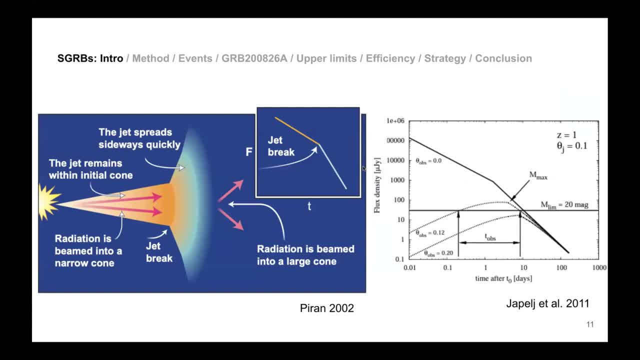 Then, basically, this was to tell you that there are a bunch of things happening within this explosion. As you may imagine, this material is traveling And since it's traveling, it will encounter this new matter in the environment and then eventually will slow down. 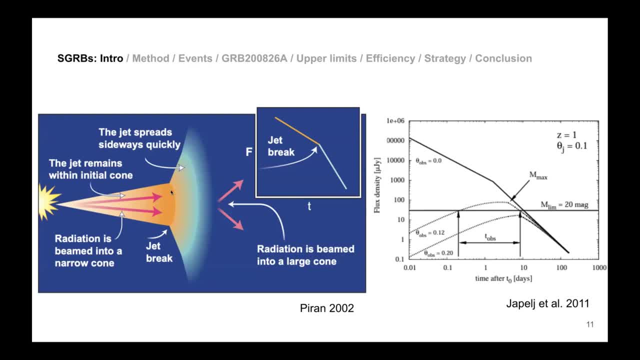 And as it slows down the radiation also changes. So you have what is called a jet break. that will occur when the Lorentz factor drops in order of magnitude, So basically when the material slows down, That produces that the radiation is less beamed. 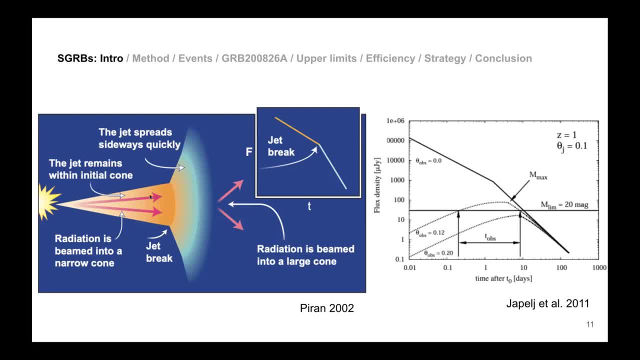 So you have here a very collimated radiation here. But when it slows down it starts to emit in a wider area. So then you have less photons, So then the brightness of this afterglow will drop. So you have here what we call a jet break. 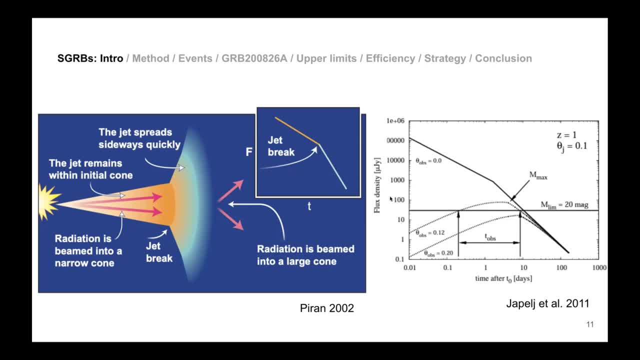 Here are more scientific simulations. This, depending on where you are, you will see different things in terms of what if we're looking right through the jet? Basically, what if the observer- yeah, the viewing angle- is 0. So we will see something that is fading very fast. 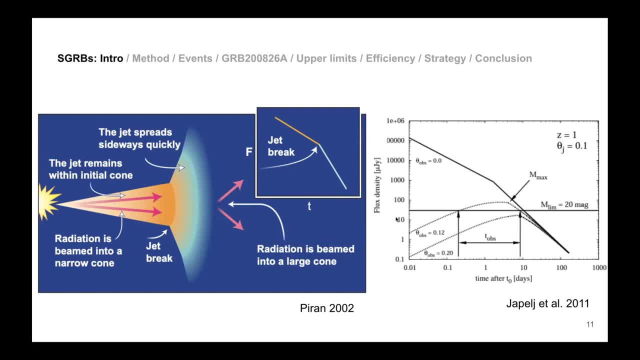 And then you have the jet break here and it goes down. But what if you're somewhere outside of the jet? So what if you missed the first part of the afterglow? So you don't really see anything until you start seeing something. 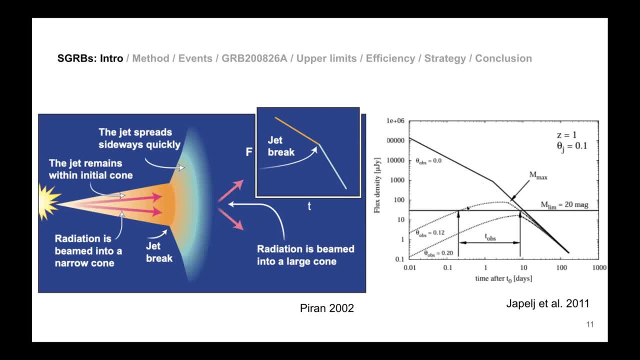 And then you start seeing something, but you don't really get that much of the energy. So eventually, when the jet breaks, you will start decaying. So depending on how far you are from the center of the jet, you will see different things as well. 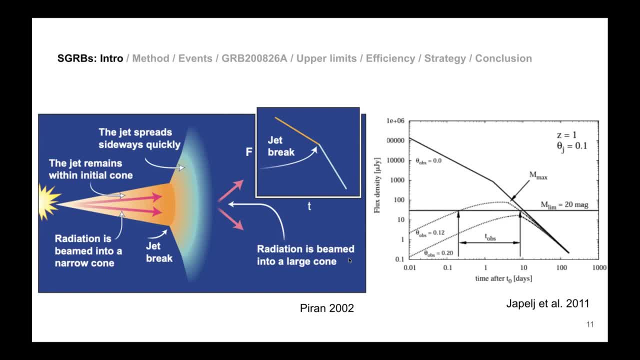 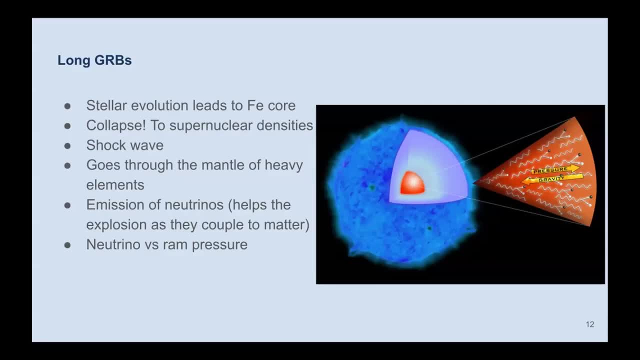 So, again, this is just to show you that the phenomena that is happening behind what we see can explain what we actually see. I'm going to take a little detour and explain what are long GRVs, because it's a little bit relevant to what we've done with CTF. 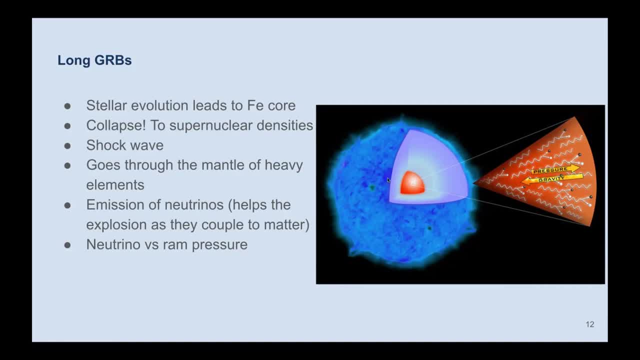 So you have here- remember that I showed you a number of progenitors. I'm just going to focus on the one that produces long GRVs. So you have a massive star that, in the center, eventually leads to the production of iron, And there's this gravity versus pressure. 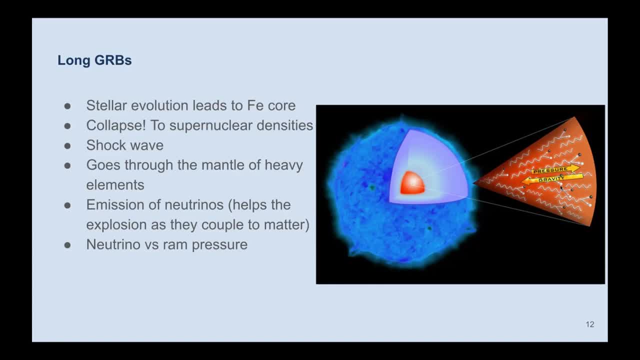 It's a very linear sort of game And eventually gravity wins. Everything collapses. We undergo this super wave of nucleotid synthesis because the nuclei collapse, And then you have these shock waves that are going through the material and are producing new elements. 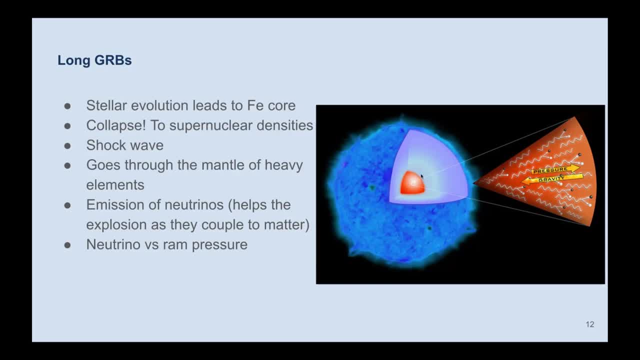 And then this material would immediately meet a lot of neutrinos because it's undergoing nucleosynthesis, And these neutrinos help explode the star. That's what basically powers the supernova. So you have this new balance that it's instead of the pressure that comes from the nucleosynthesis. 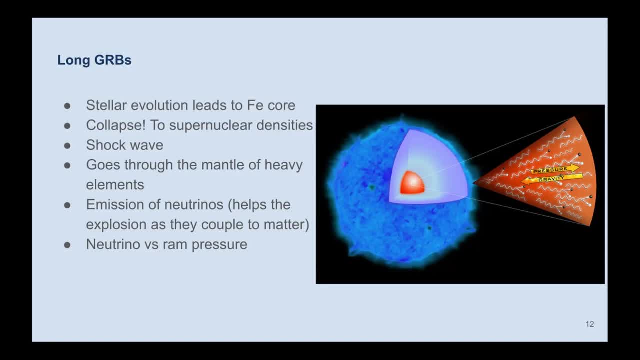 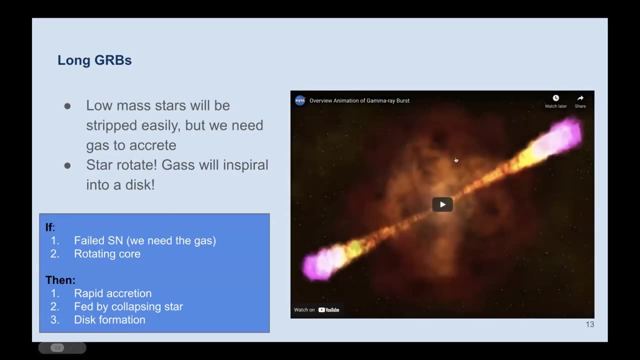 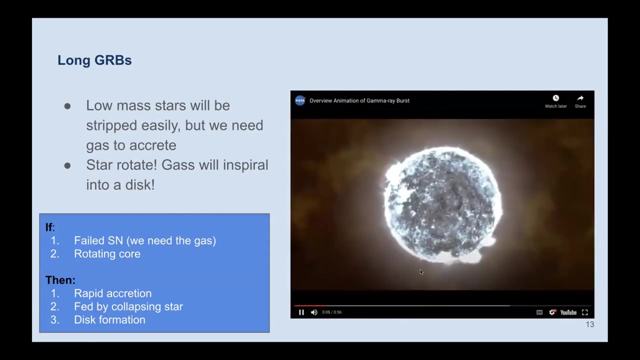 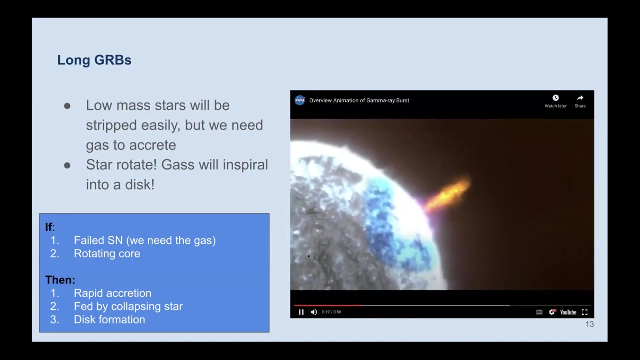 in the nuclei you have the neutrino pressure that is going and exploding everything and pushing everything out versus the pressure of the material itself. So sometimes I have a little video. So you have the center, You have a massive star And in the center you have the collapse. 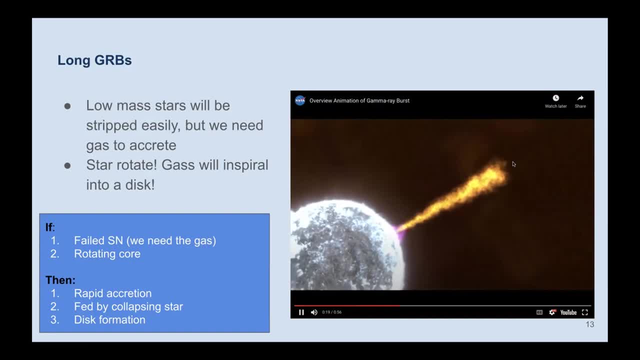 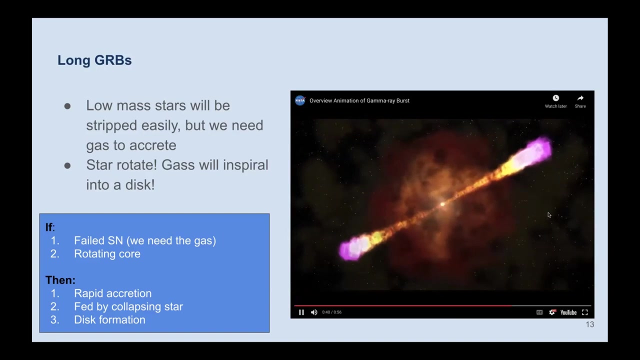 This is the jet that breaks through. It's going very fast And eventually it will collide with the material that is around the star And that produces the afterglow that we talked about. So the thing is depending on where we look at. 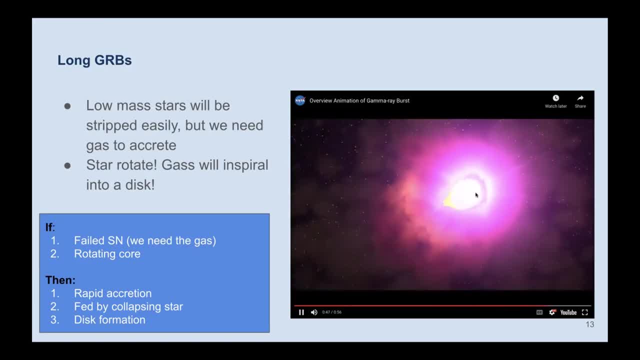 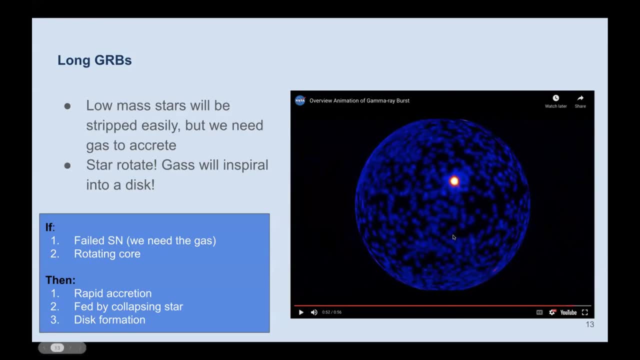 we'll see different stuff. So if we look directly through the jet we'll see the gamma ray, like that, But if not we'll be able to see part of the afterglow. So some characteristic of these long GRVs. if you have to produce this long GRV, 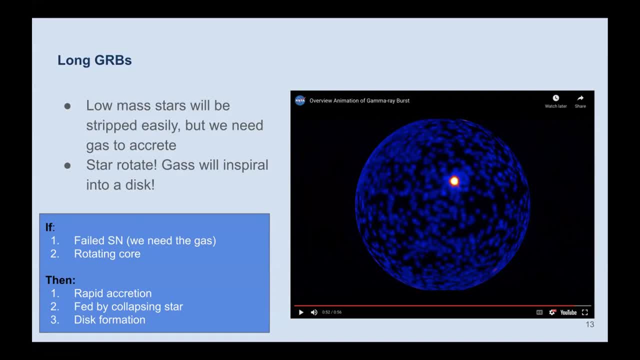 you need gas that is accreted in the black hole that is created right Right. So when you have this neutrino expansion, if you get rid of everything, you're left with no gas, And that usually happens with low-mass stars. 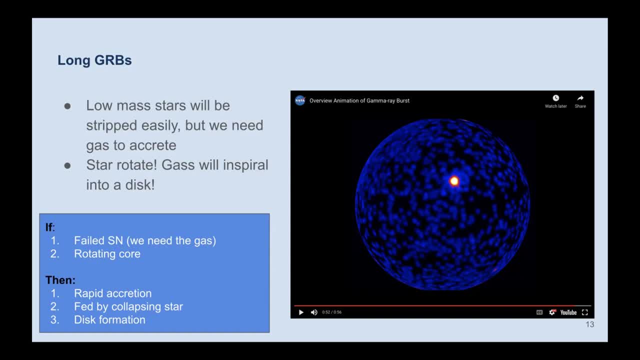 Low-mass stars, they easily lose all their gas. So then there's nothing to accrete and then there's no GRV. So we first of all need something that is massive, So the neutrino flux that it's creating, right. 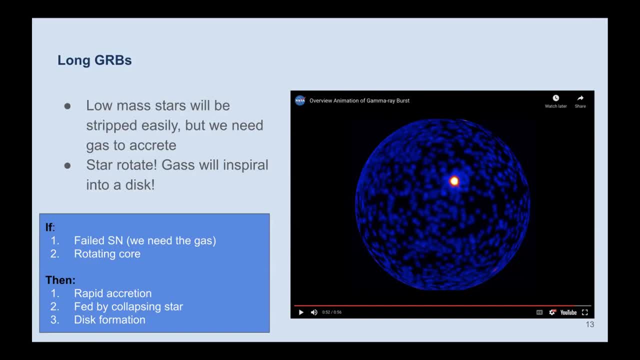 Right, Right, The flux that it's going out. it's not able to strip it off from its gas. And then you need something that is rotating. So you need a star that's already rotating, so that it comes from some angular momentum. 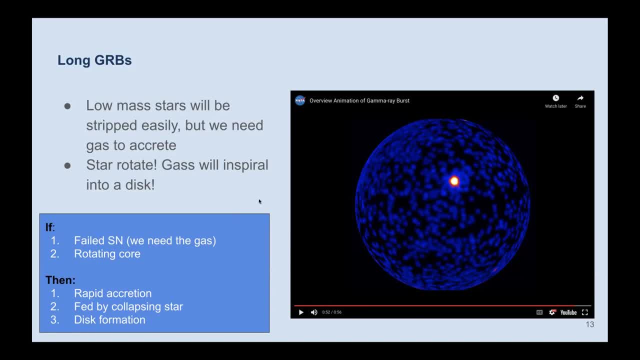 and you are able to create the accretion disk. So if the supernova fails, so if the supernova does not explode and leave everything behind, meaning, you know? meaning that there is some gas still around, and if the core was rotating already? 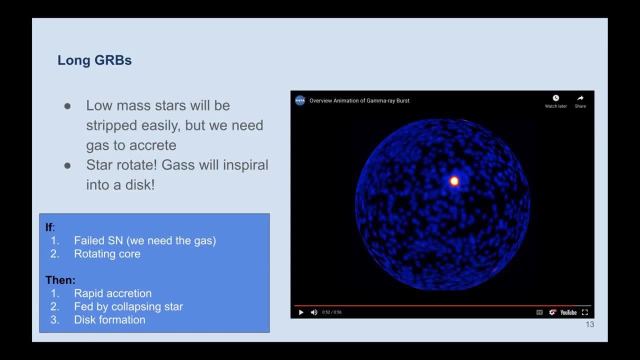 you can produce rapid accretion that is fed by the collapsing star, And then you form a disk, and then this disk will form the jet, and then you have the long journey. So that's the recipe, basically, And that is called a collapsor. 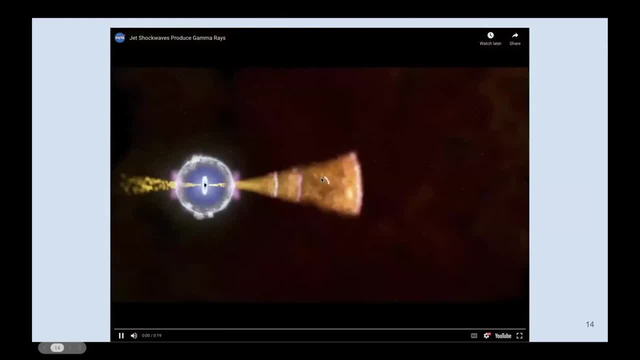 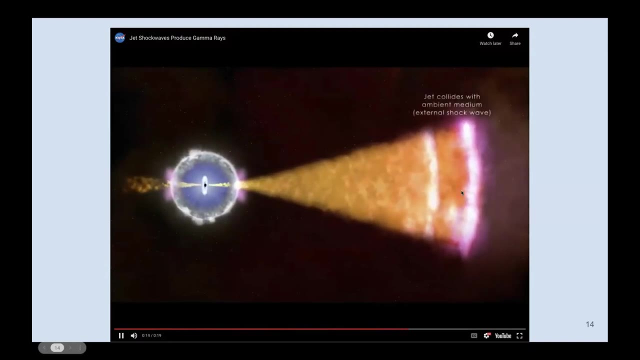 That's the collapsor model. It's another little video, And what is produced after. so you have the black hole engine that is accreting and then you have the jet, You have colliding material. That's what produces the afterglow. 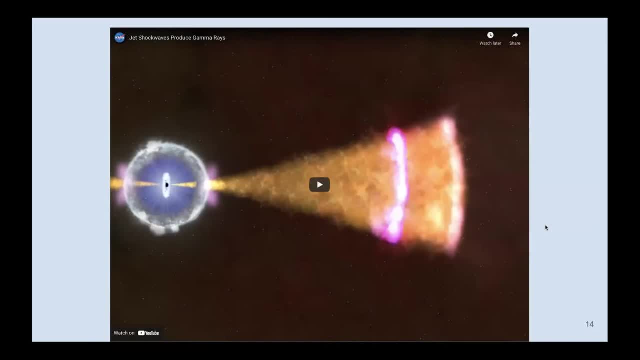 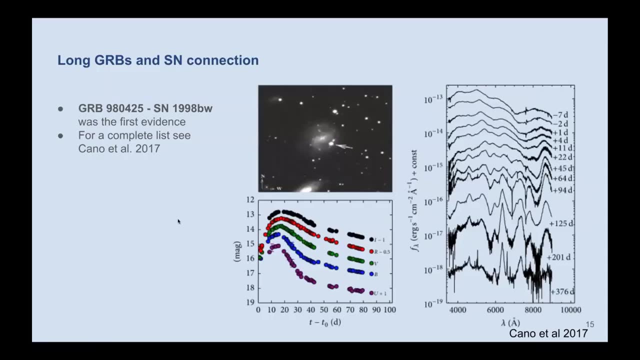 So that's basically what we are looking for. Then how do we know this? So there's a lot of history behind it, But basically the first evidence that we have it's the GRB. that happened in 1998.. So you have the name of the GRB is. 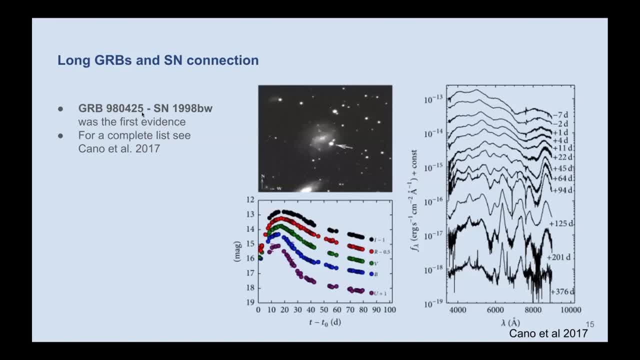 98, because of the year, 04, the month, and then 25, the day. That day we observed this GRB And a few days after we observed the rise of a supernova in a galaxy. So you have here a galaxy and then you have here a supernova. 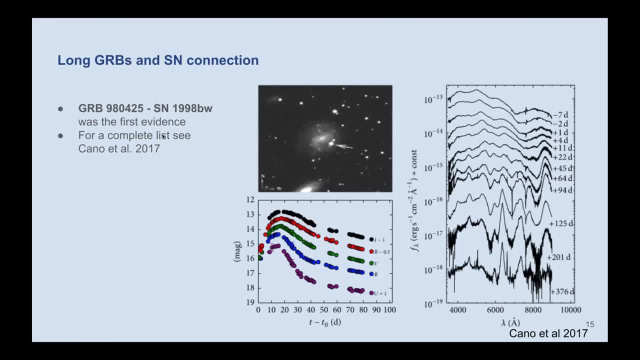 And you can monitor the supernova optically. Remember that supernova events last for days, while the GRB just lasts for a few seconds. So it's kind of hard to do the one-to-one correlation, But since we have seen a bunch of them together, 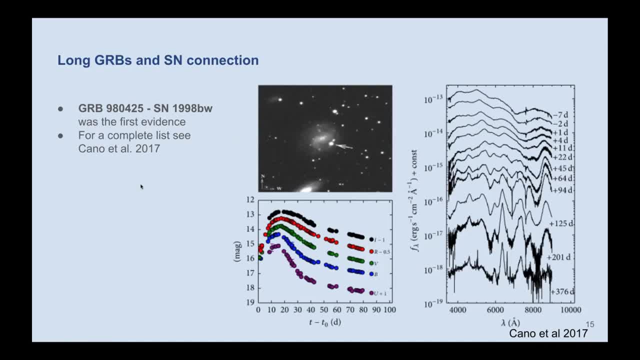 it's fair to say that it's a good thing. I just wanted to say that they are basically produced by collapsing massive stars. There is a special type of supernova associated with long GRB, But I just wanted to say that there is a supernova connection. 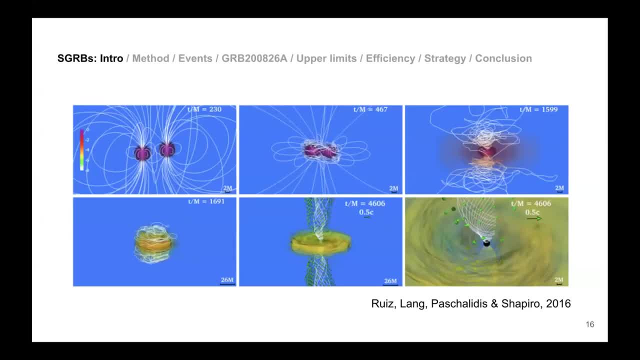 to long GRBs. Then we have what we're actually interested in, that are short GRBs. So here is just a picture of a theoretical paper. So theorists, What they usually do, they simulate physical conditions. So it also took me a while to understand. 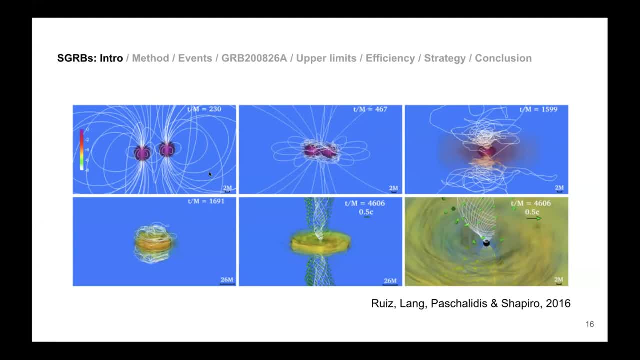 when I was an undergrad. how would this happen? So they just use computers, which is something like computers. what are they? So you have here two neutron stars, You have here the magnetic fields around, And then, when they merge, they start. 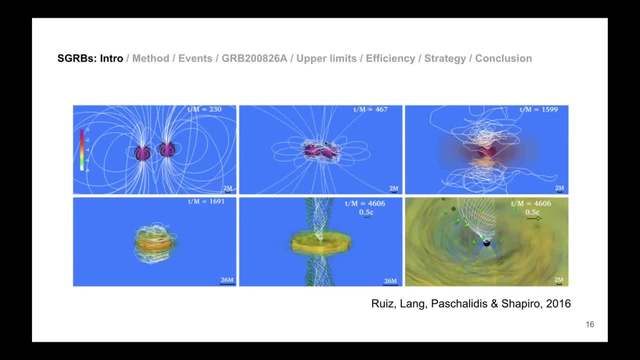 mingling their magnetic fields. It's then a mess. So you see here- I'm pretty sure that you already talked about kilonova, but we're going to talk about that too. Then you have here the tidal material that is expelled before the merge. 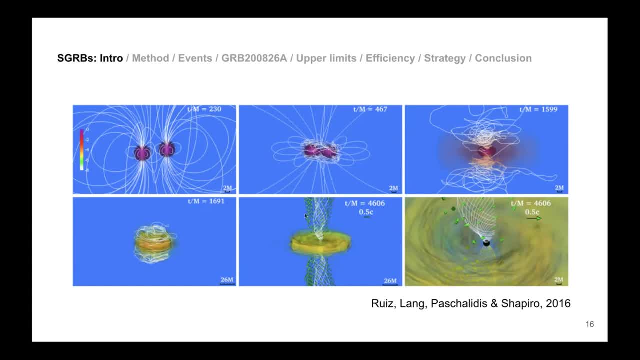 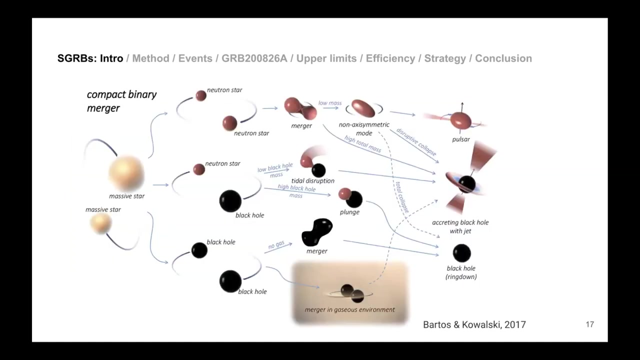 And then you have the actual merger here, And eventually this will produce a structure in the magnetic field that will allow for jets to happen. So the whole point of this slide is that No Neutron star mergers can produce jets, And when a jet happens, we know that an afterworld will come. 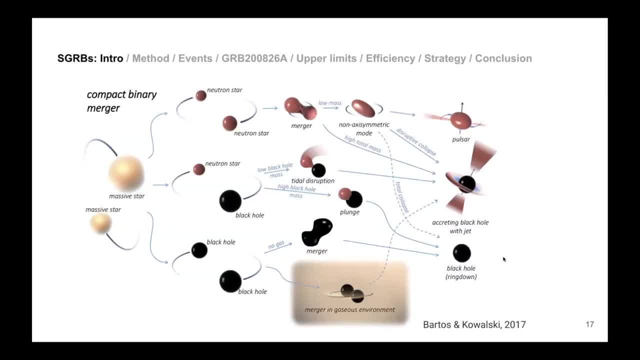 There are other objects that can produce this sort of jet. So you have two neutron stars. here. You have a compact binary merger. You have two massive stars that eventually evolve into either a pair of neutron stars, a neutron star in a black hole, or a pair of black hole. If we start with a neutron star, we'll get a neutron star. We'll get a neutron star in a black hole. We'll get a neutron star in a black hole. We'll get a neutron star in a black hole. But if we start with a pair of neutron stars, when they merge, they have two options: They can produce a bigger neutron star Or they can just collapse into a black hole. If this collapses into a black hole, you have material accreting around the black hole and then you produce the jets. 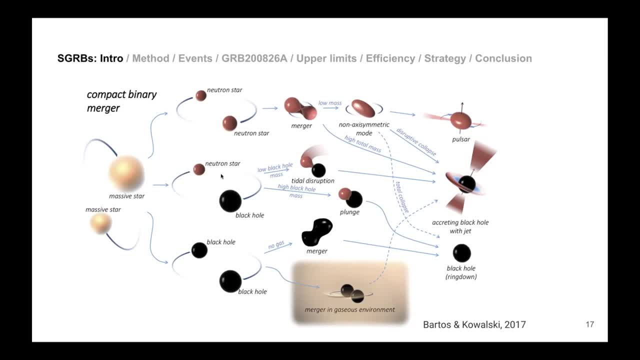 Then similar situation with neutron star in a black hole. If the neutron starts, it can also be just swallowed by the black hole. But if that doesn't happen, if there is tidal disruption, you'll have an accretion disk And then you have jets. 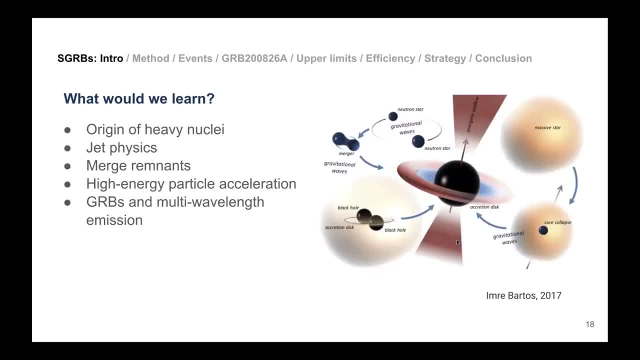 And then if you have jets, you have an afterglow. Then I just wanted to let you know that with those, if we found those compact binary mergers, honestly we haven't- we're able to unambiguously say that this is a binary neutron star. 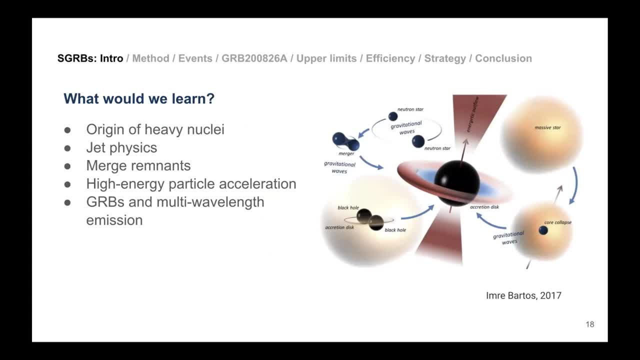 merger for 17.0.17.. It's really hard for other sort of events to say yes, this is a binary neutron star merger, But if we were able to say to find more, we could study all this, basically all these properties. 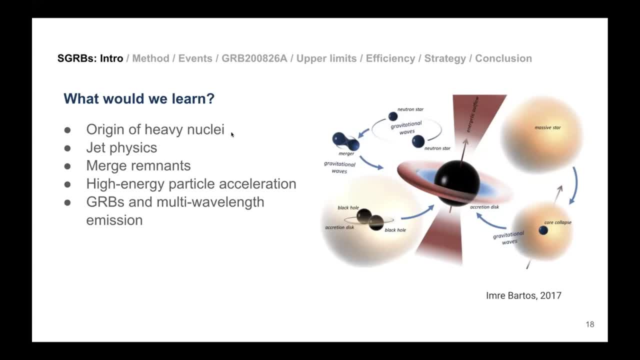 So you have the origin of heavy nuclei. You have jet physics. That's because we have jets in the in the picture. We can study what remnants are left behind. We can study high energy, particle acceleration And basically all the electromagnetic signatures. 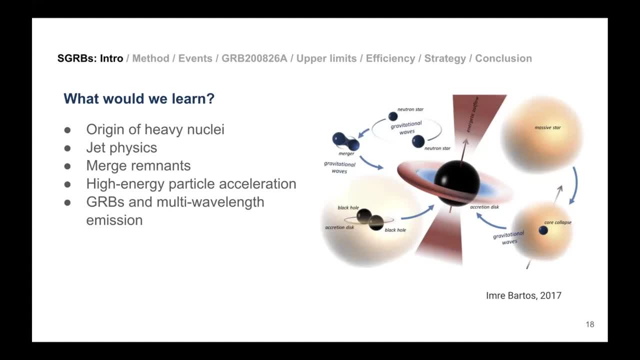 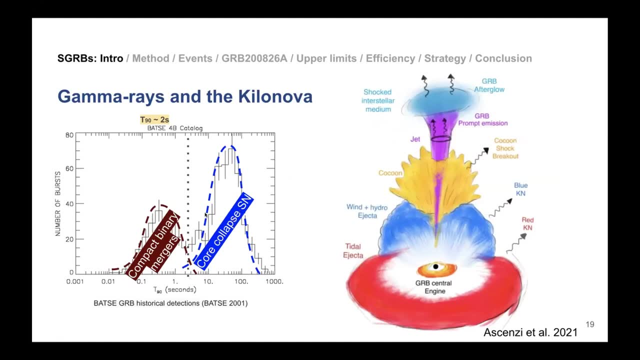 that come with this sort of merger. So, coming back to the picture, you have gamma reversed. We know that the long GRBs are produced by core-clad supernova. We know that the jet you know is that produces then an afterglow and a supernova. 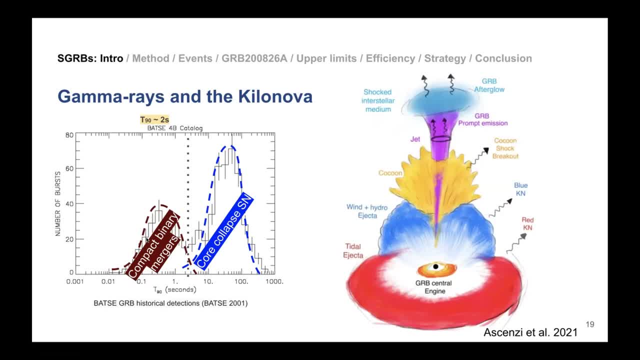 And we're going to describe now what is what happens after the neutron stars merge. So you have here a picture in which, as you remember, the two neutron stars were first tidally disrupted. So you have sort of like a cloud of material. 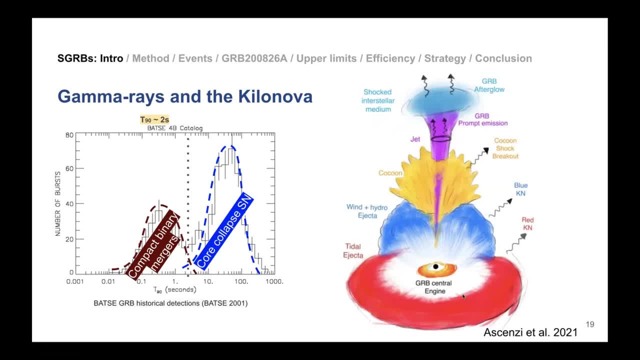 that surround the disk of the neutron star, And then you have the of the of the black hole that is generating this, that is heavy in in neutrons. These neutrons will eventually decay And they will produce radiation. These neutrons will also start bumping into one another. 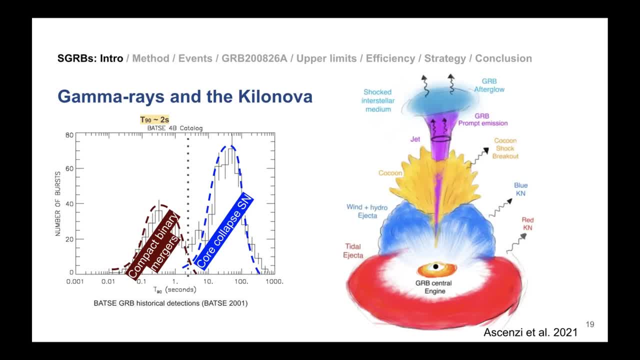 And that that will produce heavier nuclei. So we have this word core-clad supernova. So we have this word core-clad supernova. So we have this word core-clad supernova And it's a part of the periodic table. 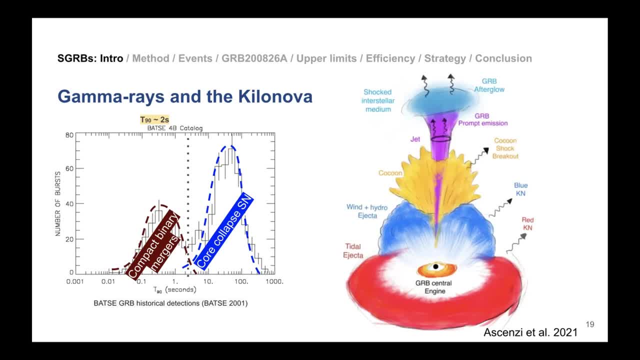 that can easily be explained with rapid capture of neutrons. So you need an environment in which you have a lot of neutrons, and what better than a neutron star? So in this situation, in this sort of red and blue cloud, here is where you are going to produce those elements that 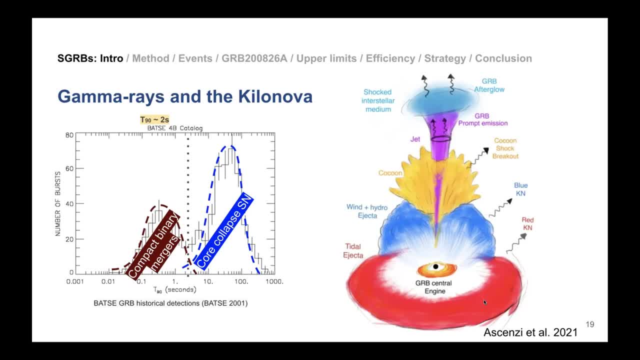 are eventually going to decay and produce the kilonova radiation. So here you have the central engine, you have the jet that we already talked about, You have the afterglow, which is the interaction with the, with the material around this structure. 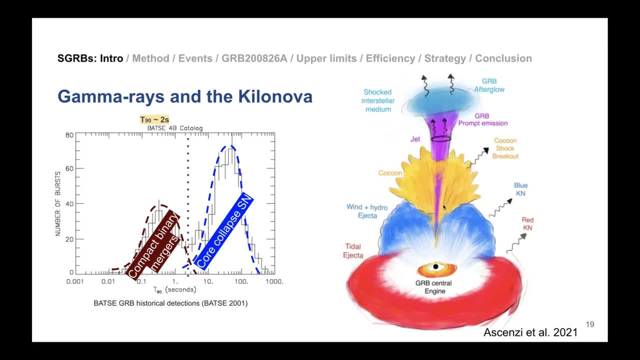 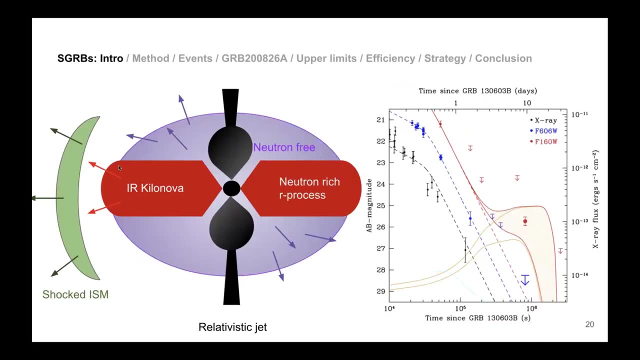 We're going to ignore this cocoon, But then we can focus on this kilonova, which is basically the emission that is powered by the radioactive decay of the elements that are created in this, in this situation. So you have here basically just wanted to show you that the the way that we, that we discovered these things in the past. 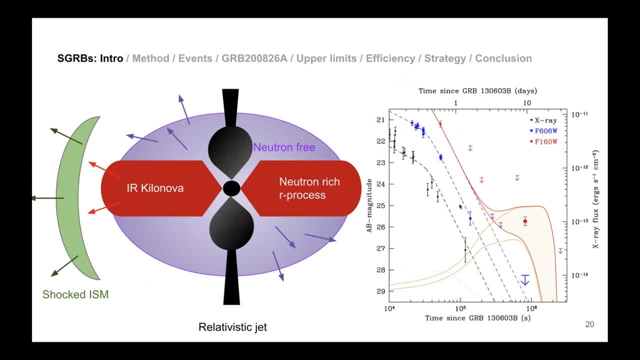 for example. this was the first one. It's basically using observations and saying, okay, this does not fit what we were expecting. So here you have GRB 1306303B. So here you have GRB 1306303B. 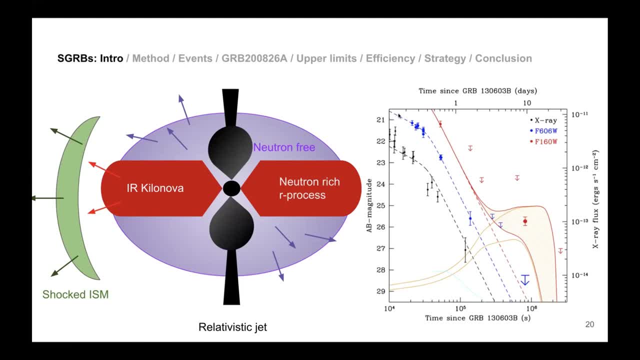 So here you have GRB 1306303B, You have here the afterglow that is in in those dash lines And then, for example, if you see the this red line, you have the observation here, And then you have that. 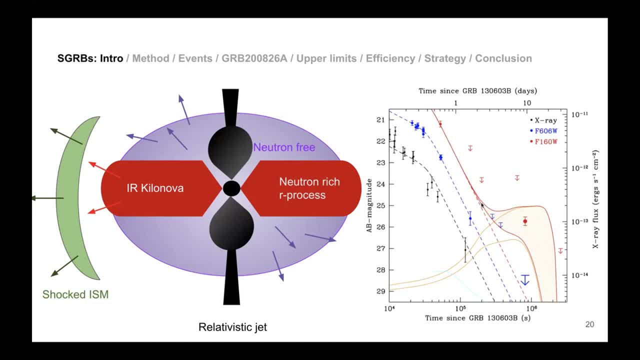 If this is just an afterglow, it would only just decay. It would decay and decay and decay. But it didn't do that because a million seconds. there was another observation that showed that then the source was brighter. so the question is: how can you explain that in such short? 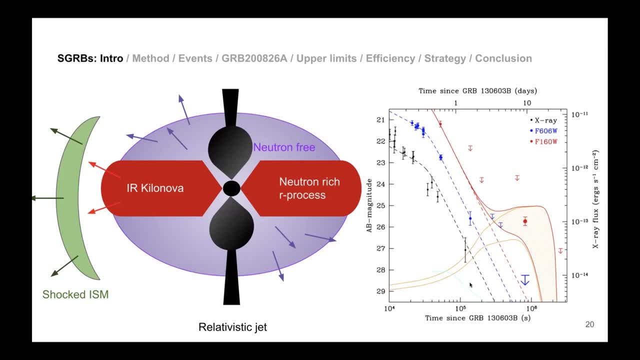 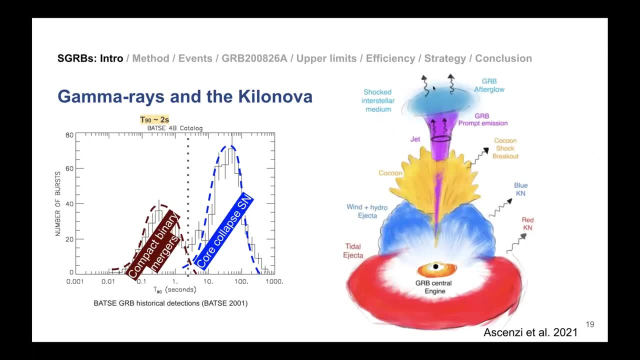 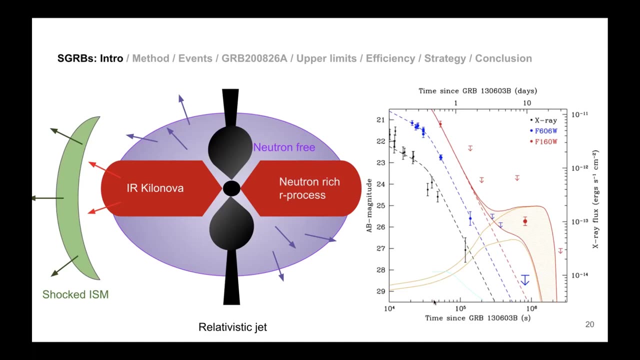 period of time. so that's when you invoke kilonova, because you have here the emission of the of the afterglow that is rapidly decaying, but then on top of that you can sum the emission of the of this kilonova. so this is the first claim of kilonova detection. 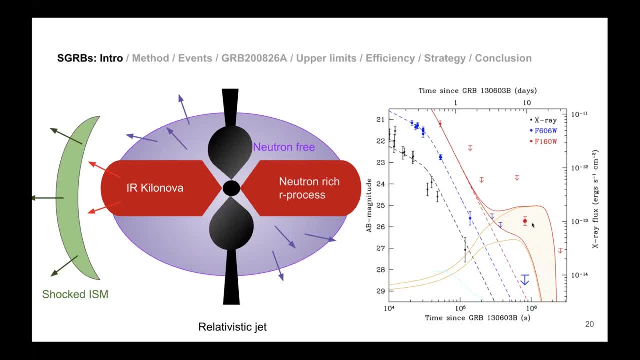 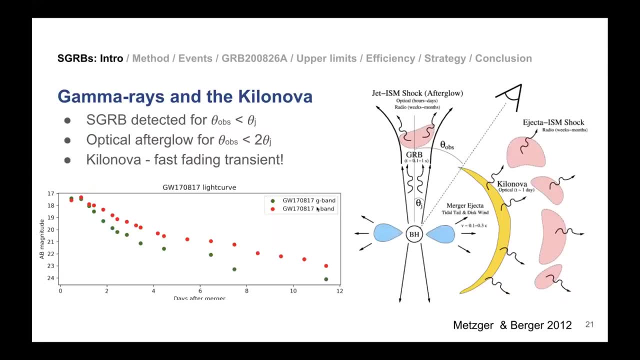 um, that is based on that one data point, so, and that was a nature paper, so they just have one data point that made it a nature paper. then, um, the entire picture then says: okay, if we are looking into um compact binary merger, depending on where we look at, we're going to see different things. 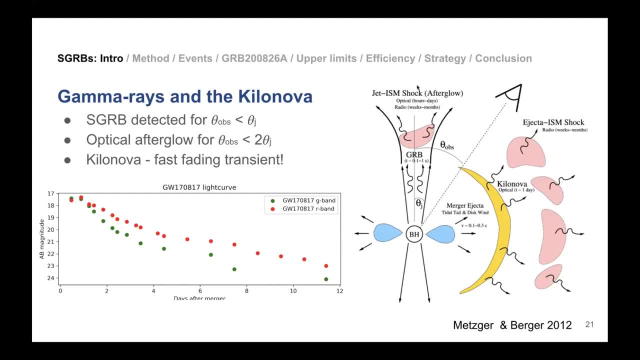 if we look through the jet we're going to see a grb. if we're not in the jet, if we're like slightly off, we're not going to see the jet, but we will see. the optical afterglow of it could be also x-ray. 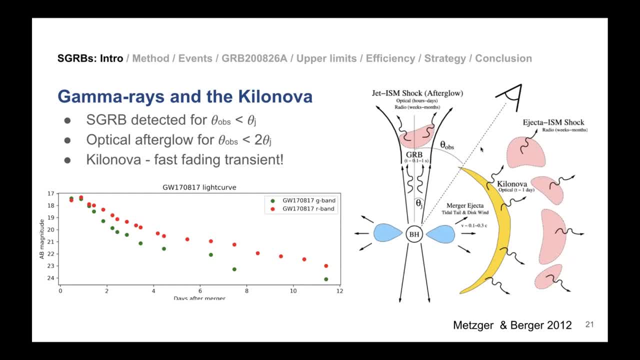 and, and and in radio, because, as i told you before, this um it's non-thermal emission, so it really it's in the entire spectrum. so, um, but even if we're, even if not, even if we're farther away, we should be able to see, uh, the kilonova. so the kilonova is also very fast in in nature, it's a fast. 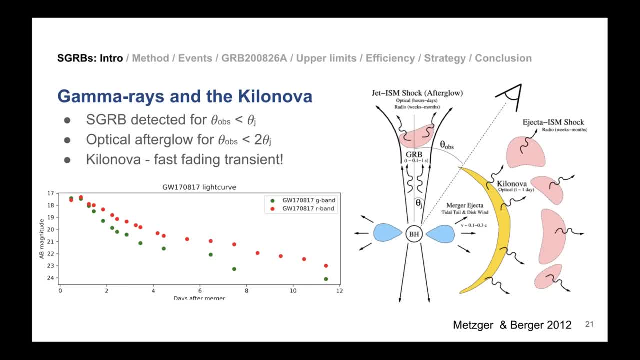 straight, uh, fast fading, transient um, and i'm sure that igor told you everything that you need to know about um than yesterday. so this is the light curve of 1717. you have um that it's kind of like magnitude 17 and in less than two days goes to 19 and a half. so it's a very, very fast fading. 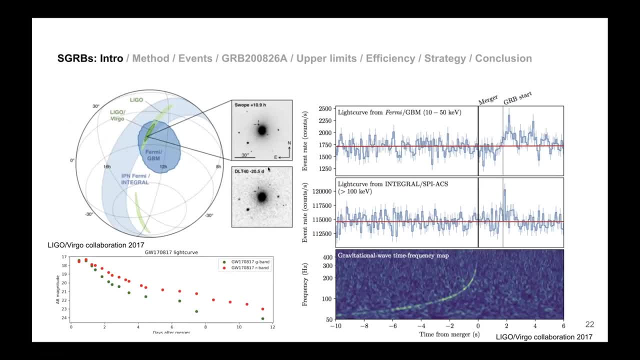 transient, um. you have here, um basically now is the motivation for my work, which is trying to look for um more of these binary nutrients are mergers. so what do we do? we know that this um, this is the lego localization map, this is a gravitational wave, um, basically map um. and we know that um from 1707, um when two 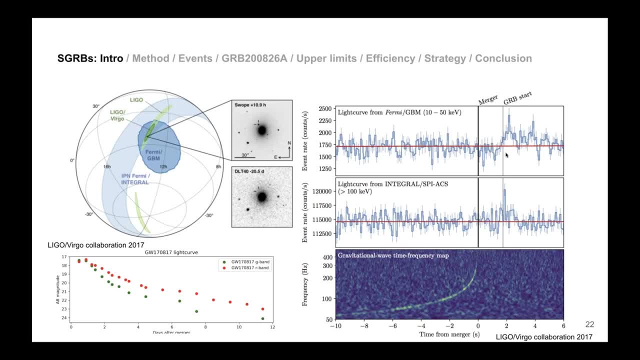 stars. two nutrients are merged, they will produce a short gamma ray ray. so here you have the gravitational wave time frequency map. so you see the frequency going up because they're going faster and faster, so that the frequency goes up and eventually they merge. and then you have two. 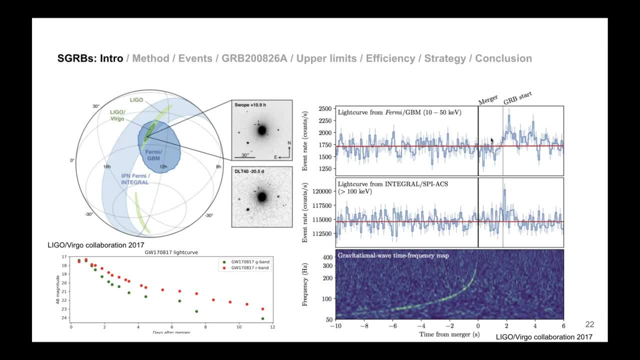 light, two grb light curves. you have the fermi gbm- that's another instrument- and you have um in in another spacecraft and you see that after almost two seconds um you detect a short grb. so what if we go after them without the gravitational wave trigger? what if we just go and look for optical counterparts to short grbs? 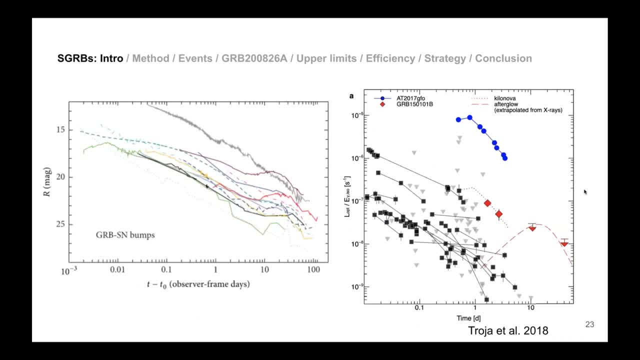 and that's what i've been doing, um, but i have found it very hard because, um, as i told you before, there are a lot of things that could also look like um fast fading transients, for example, the afterglow. so you have here um long grbs, you have fast fading things, but how do we know that these 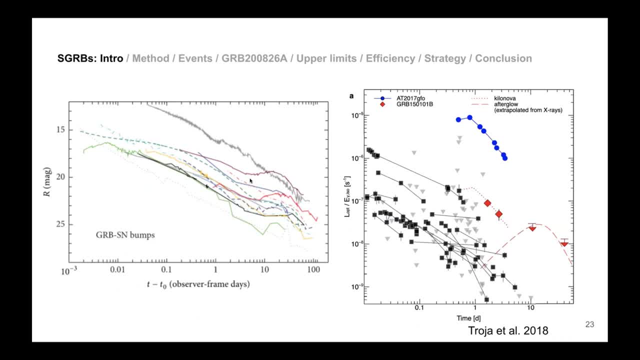 are not binary nutrient stars because they have a bump after, uh, tens of days. so this is just to show you the scale: the, the supernova, will be visible to us after tens of days, while the, um, the kilonova, um, kilonovas are visible after a couple days. so the scales are are much different. 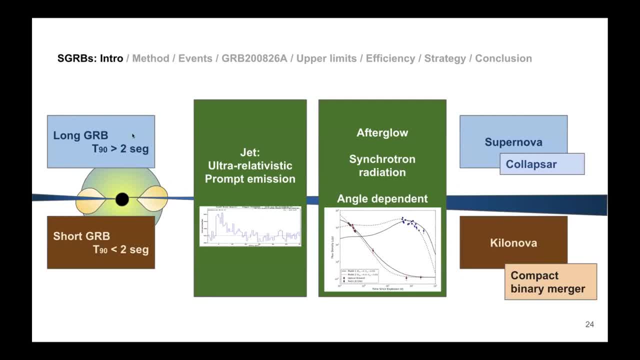 um. another sort of summary: if you have a long journey that lasts longer than two seconds, you will produce jets, um, and those jets will produce an afterglow, and then you should be able to see a supernova, and that's what we call collapser. then, if you have a short grb, you will 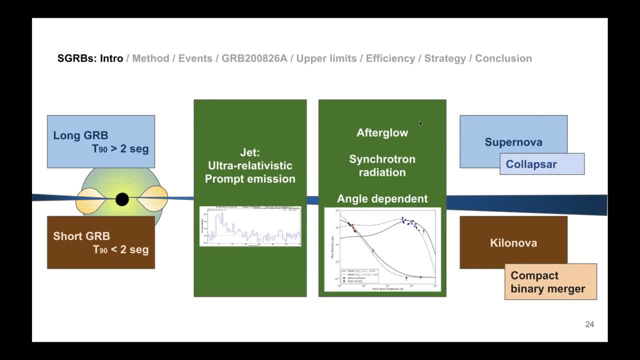 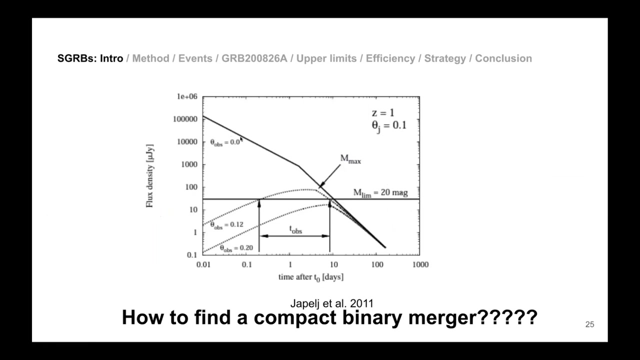 see it, that will produce jet, um, they will produce an afterglow, um, but um, the the optical would also be powered by a kilonova, um, so, um, that's, that's how we know that it's. uh, the, the origin is a compact binary merger, so again you have the fast fading. um, what if you find something here that is fast? 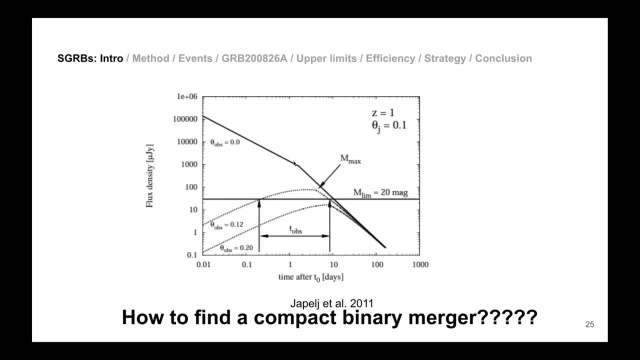 fading. what if you say: okay, this is an afterglow, the the way to to know whether the origin, the progenitor, is uh, collapsing, a massive star or a kill, or a compact binary merger, is to look for kilonova signatures in the light curve: or a compact binary merger? 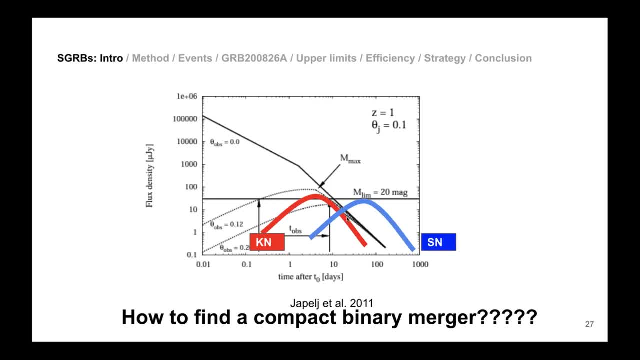 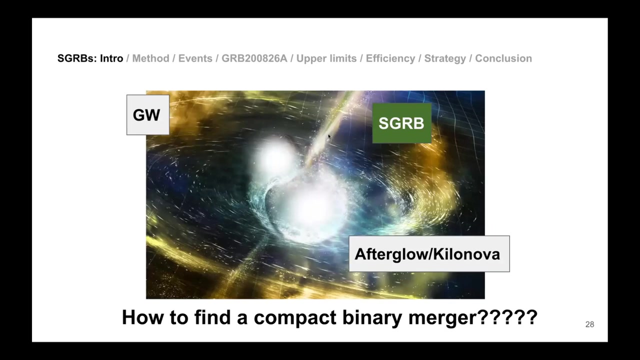 or supernova um signatures in the light group. the good thing is that supernova are much brighter than kilonova, um, and they also occur after um in time. so it's it's um. that's at least an advantage that we have in our, in our hand. so how to find them? um? shreya talked previously about. 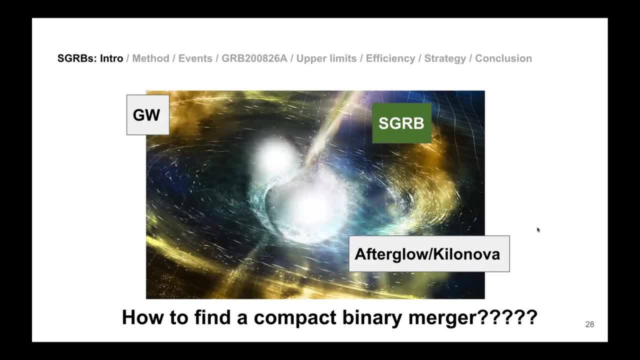 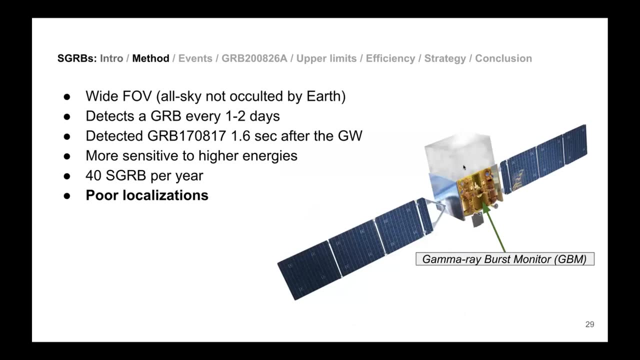 gravitational waves um. igor probably talked about how you will be able to catch the kilonova um signature without any sort of trigger, but i'm gonna just focus on the short grvs we have been using fermi. fermi is a satellite um that has. 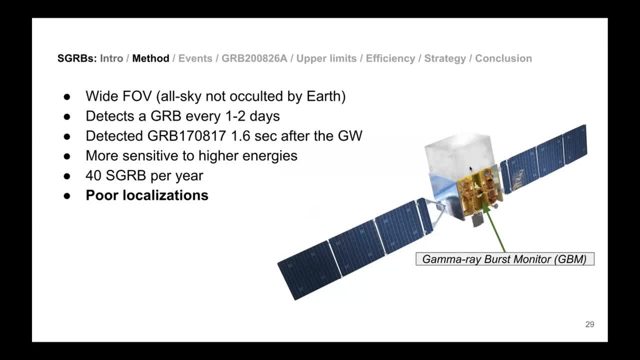 well, it's basically this one here, um, it has two compartments. the one here has one instrument that is very sensitive to high energies, like super high energy, um, but then we are using the gamma ray burst monitor. it's, it's some, some sort of, um, uh, an eye on the sky that's looking everywhere, so it has a wide field of view. it's basically. 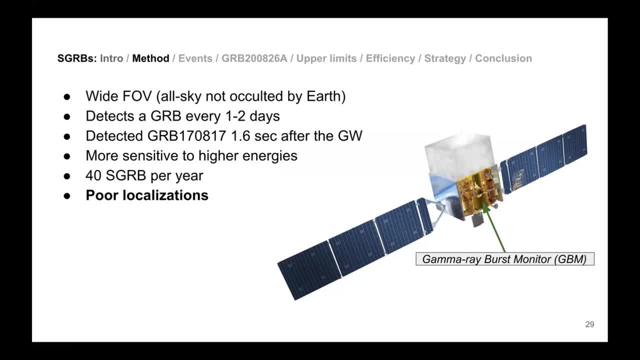 looking everywhere in the sky, uh, it detects a couple of grvs per day. um, it was able to detect 1717s and that's good because we know that it works. um, and it's more sensitive to higher energies, which is where it's shorter is 10 to a core. we have this rate of 40 short grvs, but the 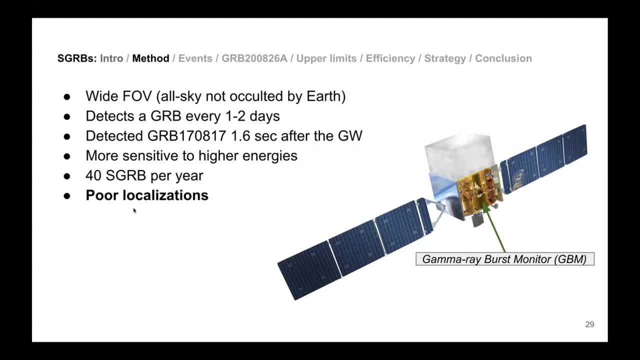 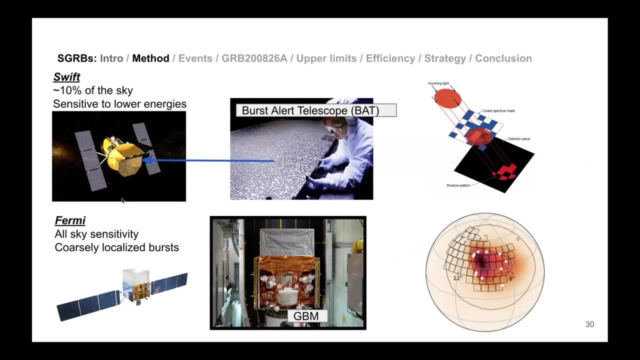 thing is, um, it's really hard to locate them. so these are eyes that are just looking everywhere, but it's very hard to pinpoint where it happened. this is different from other spacecraft, um. most of the knowledge about short grvs um today comes from swift, so it's this other satellite. 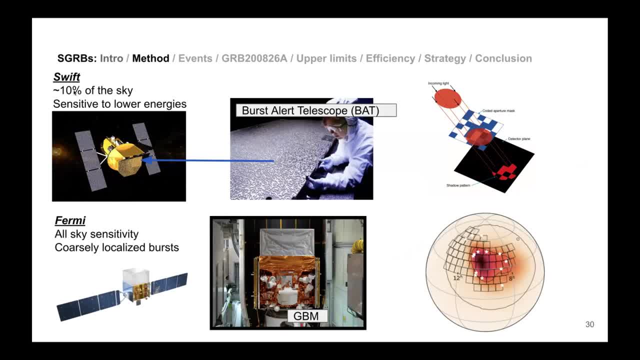 um, it is sensitive to lower energies and it's also looking into a 10 of the sky at the time. so, uh, as you can imagine, the rate of um short grvs is much lower. so we don't have many of them, um, and it's basically because of the instrument that it's using. so you have here um the burst. 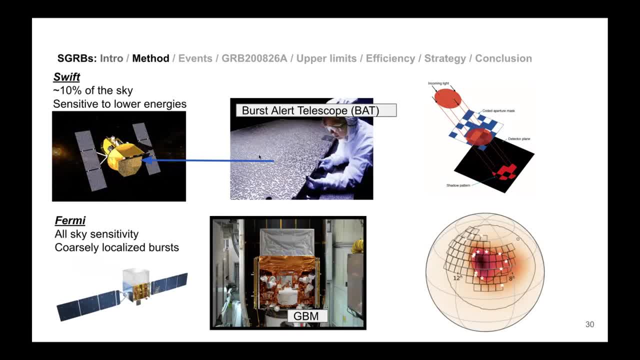 ls telescope. it's um, it's a mask of um, just those little holes that you see here. they uh, when there's a incoming light, there's a grv, they cast the shade and, depending on the, on the shadow pattern, you can reconstruct the direction of it. so that's how this one works and that's why it's so um, that's. 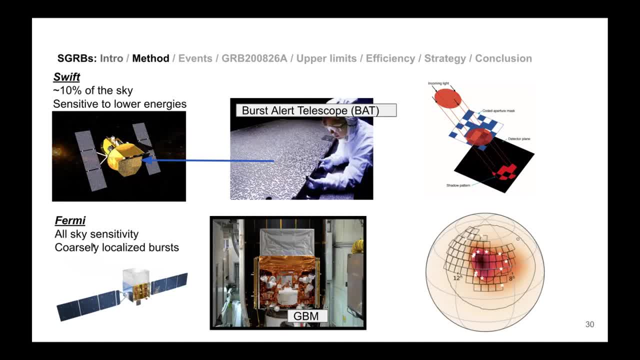 why the field of view is so small, while thermy, the one that we are using, uh, uses those little white things that are basically eyes looking into all directions. so if a photon comes from here, you will go to this one first, and then you can triangulate and say, okay, it come, it comes from. 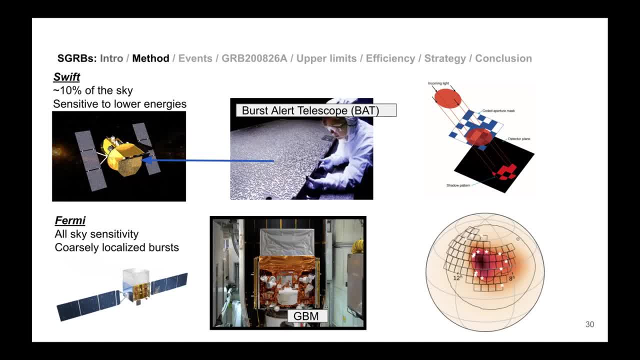 this direction, but the problem is that it only tells it sort of like a direction. here you have a localization map of gvm. um, it's pretty terrible. you have thousands of degrees and we actually looked into it and found things that were rapidly fading. uh, none of them. 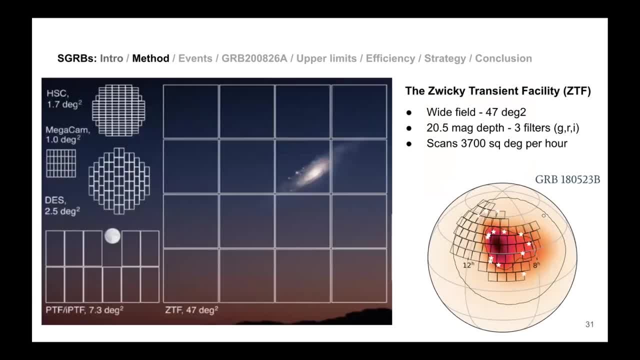 ended up being the, the short grv. but whatever, we tried, um, we're using this, the swiki transient facility, to do this. i'm pretty sure that you know about this. uh, why? because the localizations are terrible. so you have um. you need a telescope that can tile the regions very fast. so, um, you have here. 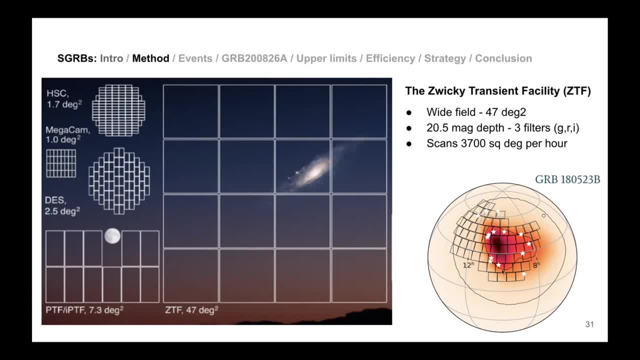 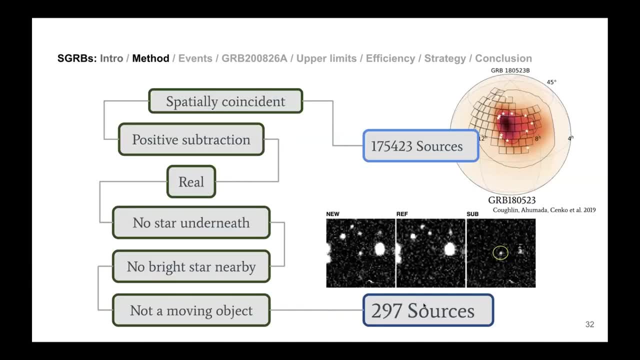 in black squares, have regions, and then you have all the stars, all the transits that we, we followed up um. how do we do this after we receive a localization map like this one? for example, we, um, we titled regions, um, and then all the transits, all the sources are changing in flux um. will um be seen as a? 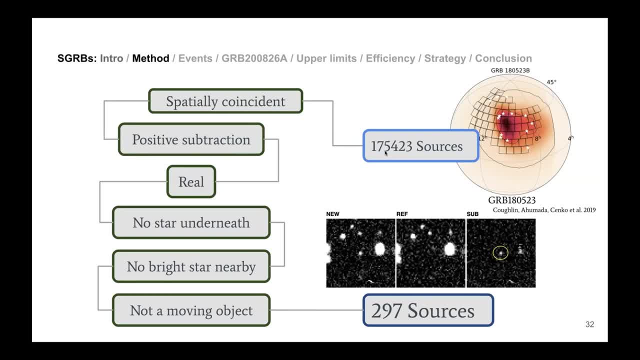 potential candidate. but then you will have a tremendous number of candidates- in this case is more than 170 000 sources, but we know that only one of them is the, the, the afterglow. so we need to run a filtering scheme. so we need that. it has to be in the region, it has to be brighter than 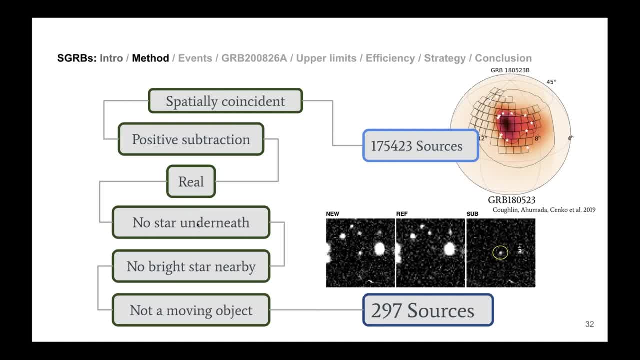 before it should be classified as real, shouldn't be close to a star and it shouldn't be an asteroid. um, when in this case, in this exercise, um, we went from 175 000 to only 300 sources, which is a little bit more manageable. we can even reduce that further if we look into the previous history of 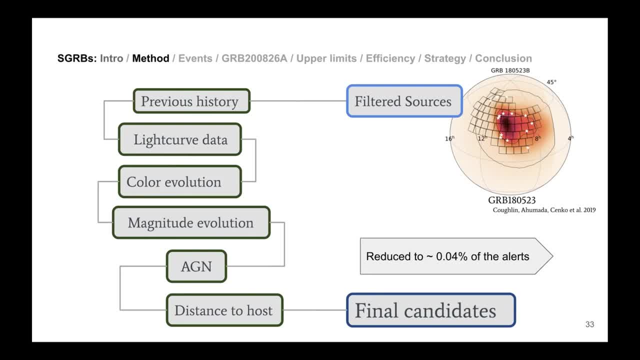 of the sources. so you look into the color evolution, the magnitude evolution, you do some cross matches with agns, because you know that those are variable sources, um, and you can also calculate distances to potential hosts and, and then you can calculate the distance to the source, and then you can calculate the distance to the source and try to reduce your number of. 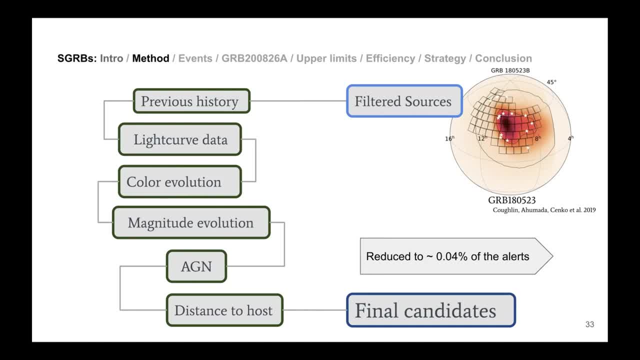 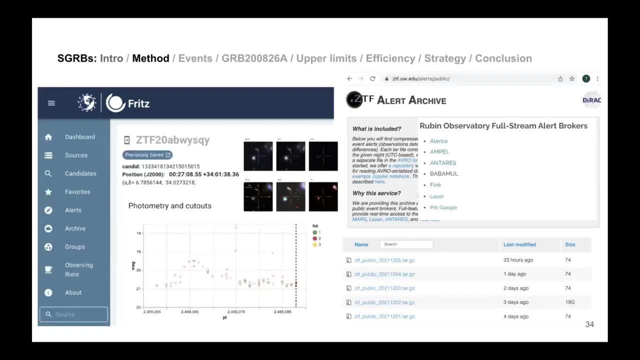 and try to reduce your number of candidates to, to less than hundreds. we usually get um, a few, a few dozens um per trigger, which is really manageable. you have here, um. how do we do this? um, we have a portal called fritz, um, in fritz, you can see the cutouts of the, of the source. 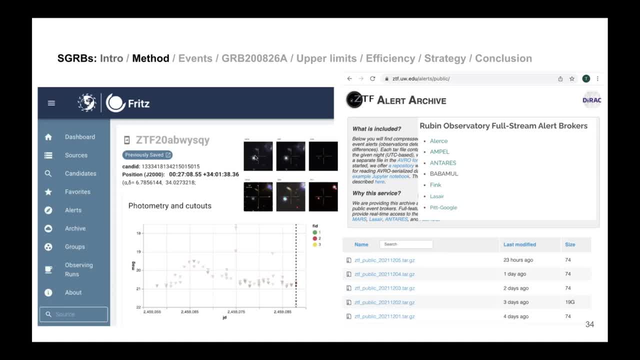 so you have um. it may be hard to see, but in the center of this image you have um, a source here that was not there before um, and it has some sort of flags associated with it. you can access this through numerous ways. you can even download the entire alert alerts discovered per night in this web page. 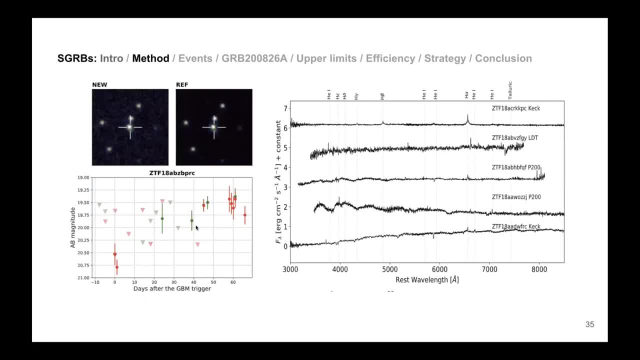 but basically what we're looking, it's for things that are fast fading. so in this case, we're looking for things that are fast fading. so in this case, we're looking for things that are fast fading. so in the this case, we're looking for things that are fast fading. so in this case, we're looking for things that are fast fading. so in this case, we discovered something that was 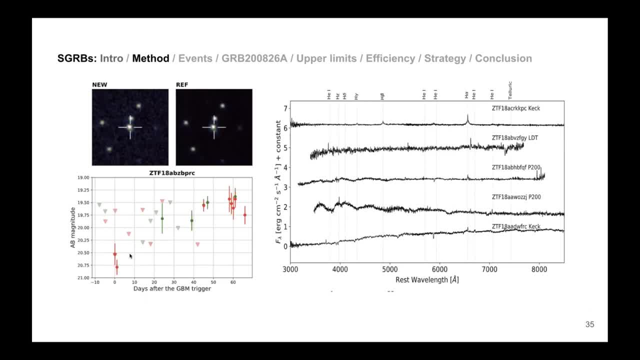 sort of like fading, but then a few days after, uh, we discovered that, okay, no, it's not really fading, it's going actually brighter. another way to to follow this up is to take a spectrum. so, um, we're looking for kilonova signatures in in the spectrum. we don't like hydrogen. 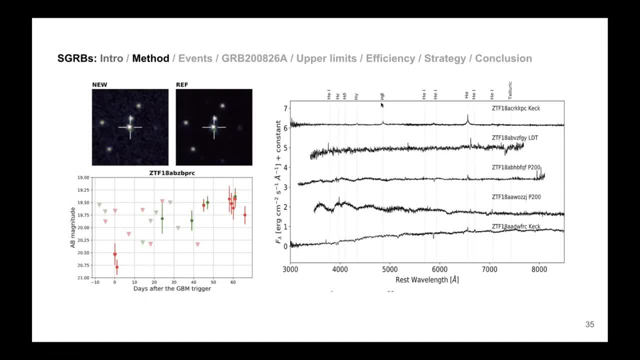 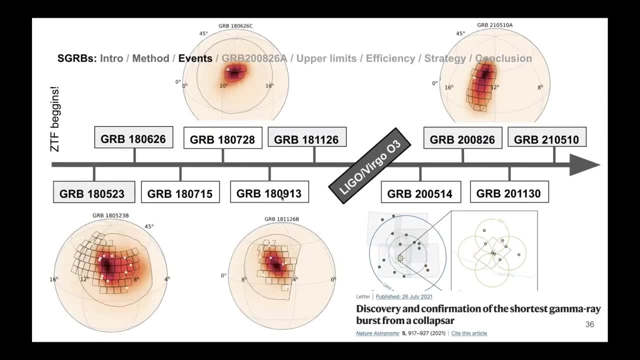 um, we don't like uh supernova features. so, for example, this one here shows hydrogen. goodbye, you're supernova, i don't care. um we've done this several times um, we actually did it six times um. we had um uh in in 2018, and then we we um came back in in 2020, because in the mid 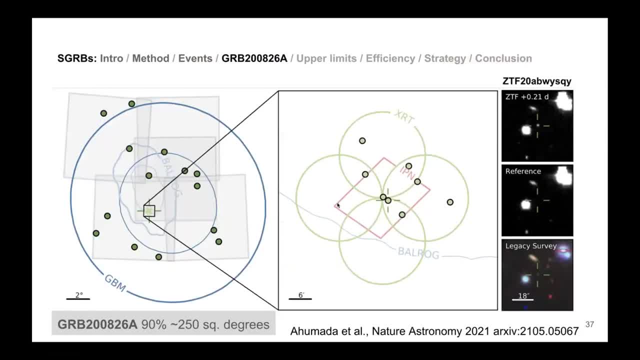 time you had the like a virgo observing run and we actually discovered something. um, this is the, the gbm localization of a short year. it lasted for about a second and and and one second and fourteen, um 1.14 seconds. and then you have here the tiling of our ctf regions. you have the. 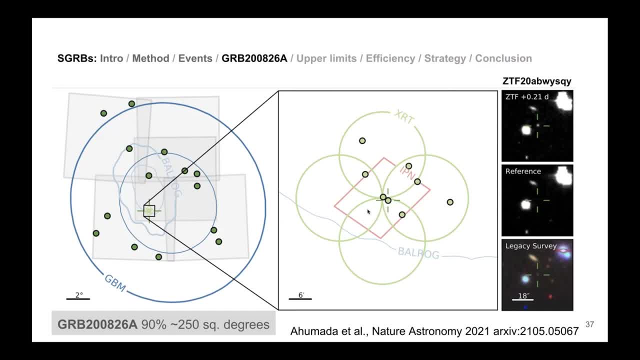 candidates that we had, um. eventually, other spacecraft um were able to triangle the region to a much smaller um localization that allowed um swift to look for x-ray variability. so those circles are xrt pointings. xrt is the x-ray telescope um. so you have um. 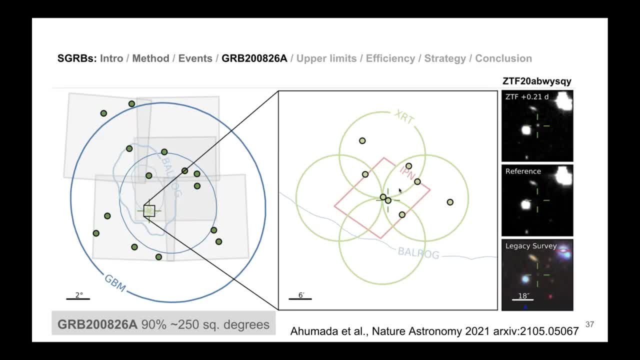 one source here, that is this one that it's variating in x-rays, but also, uh, it was a transient in ctf. so this one is ctf 20 of whiskey, this one here that wasn't there before, and there is a very small galaxy over here, a very faint galaxy over there. um, when we discovered this, we 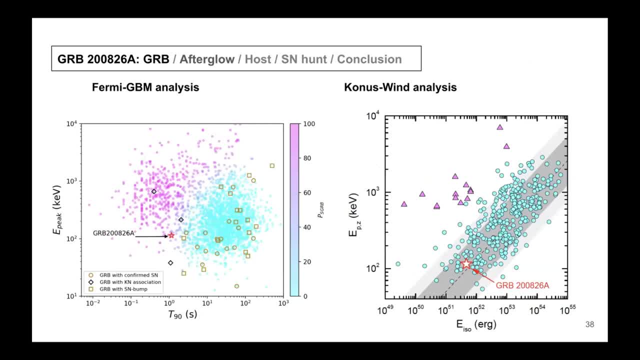 were super excited because, okay, we finally discovered a shorter v afterglow. um. what do we do now? um, since we had information about the galaxy, people were able to locate uh. put this into context with other grbs. since you know the distance to grb, you can look for the energetics of the grb. um, and, as you may imagine, long uh, the. 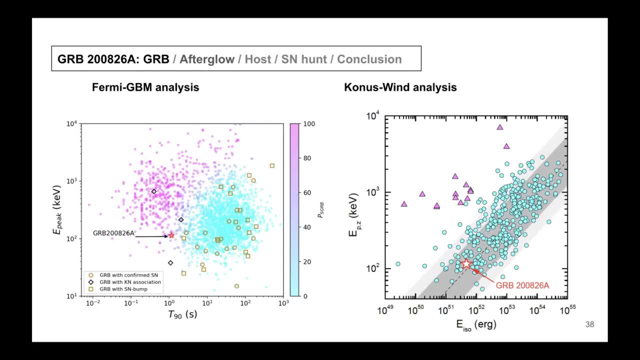 grbs that come from um, a massive collapsing star, have different energetics that the ones that come from um a binary neutron star merger. so here you have the long grb population, here in in the, in the cyan and the magenta population is the short grb. so you see that, um, our grb falls right in the. 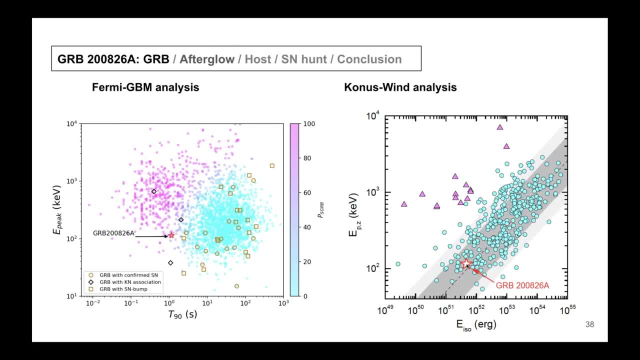 long grb population. um, so that means like it could be a collapsing massive star. um, you can do the same exercise, uh, using the duration of the grb instead of just the energetics, and in this case you also separate. here are the long jervis, here are the short jervis, and it falls. 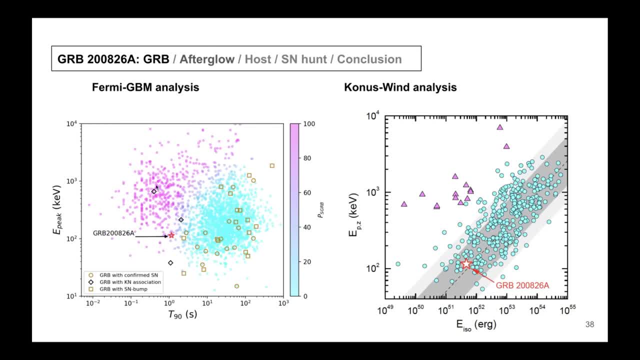 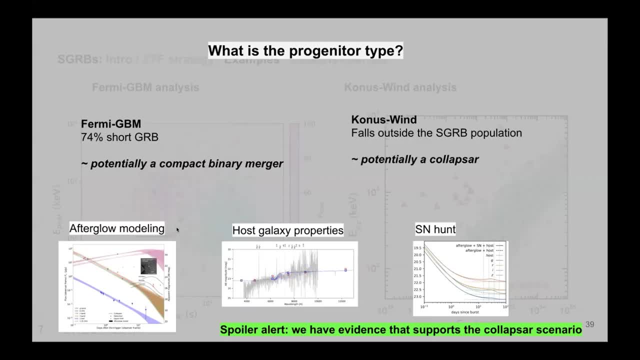 sort of like in the middle, the. the probability is not the same, so you can do the same exercise, but the problem is that the one that falls is not really 100 belonging to this population. uh, it's sort of like 74, which is basically not the site. so if you have this sort of ambiguity, 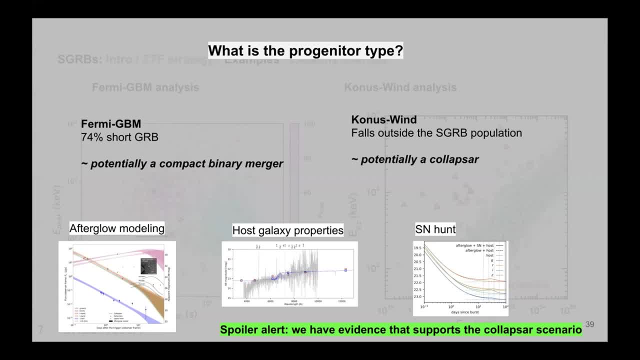 what is the progenitor type? because two different analysis say two different things. um, what did we do? we modeled the afterglow. we look for the galaxies of the? um the host galaxy properties, and then look for um a supernova and one in a supernova hand, and actually you can see that the 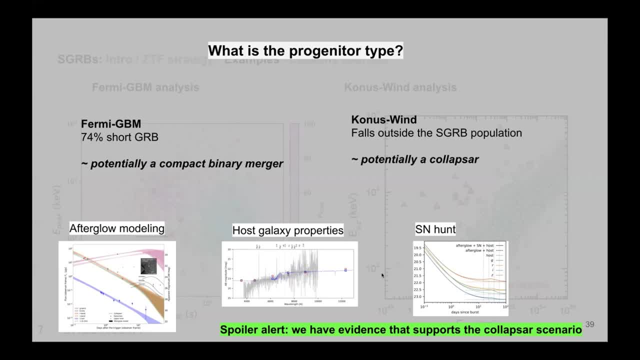 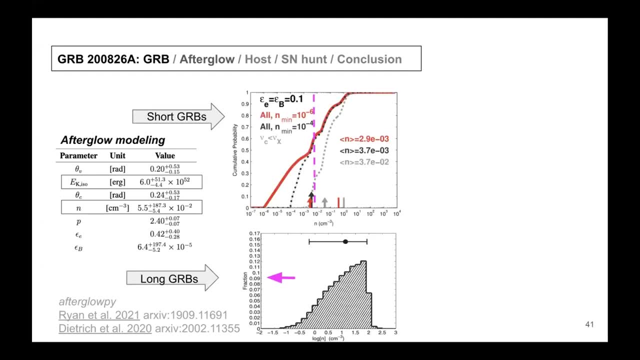 Well, spoiler alert, we have evidence that supports the scenario of a collapsing massive star. So I'm just going to start with the afterglow. As I told you before, the afterglow comes from the jet, basically, And you have two different things. 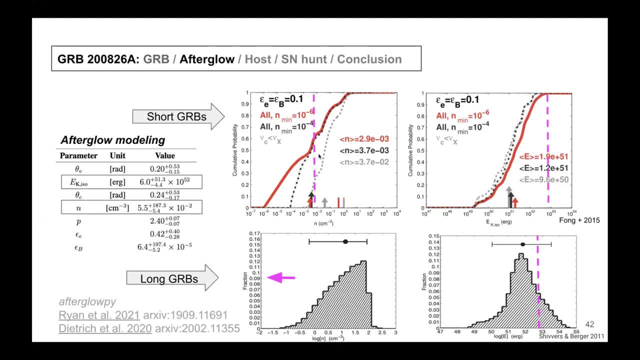 So when you have a massive star, it is expected that the density around this environment is much larger than for a short GRV. So we can model the afterglow. We have parameters like the viewing angle and the energy that was input into the circumverse material. 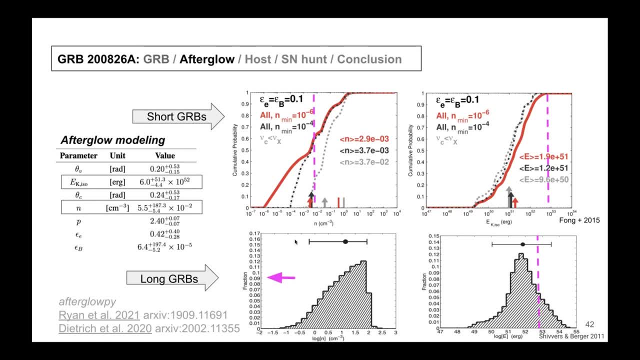 You have the density of this material. So if you compare them to the population of GRVs found you have the density That we found falls right in the middle of the distribution for short GRV densities But it's really really small for a long GRV. 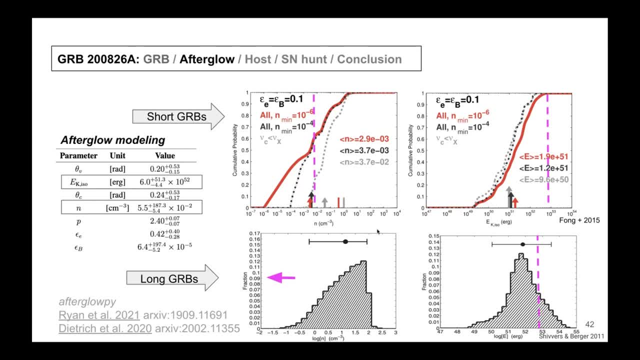 If you look into the energetics that were input by this jet, you have here that it's much higher than what we would expect for a short GRV, But then it falls right within a sigma of the population of long GRVs. So from this analysis of the afterglow, 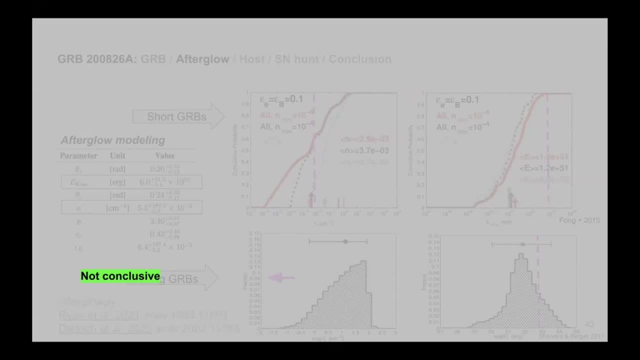 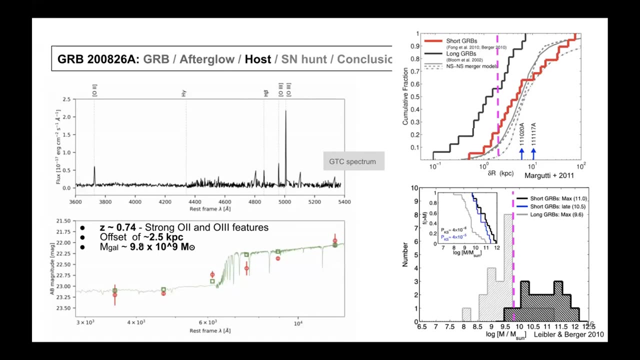 it's really hard to say what is the progenitor type. It's basically not conclusive. There are other studies about GRVs that have linked certain types of galaxies to certain types of GRVs And in this situation we took a spectrum of the galaxy. 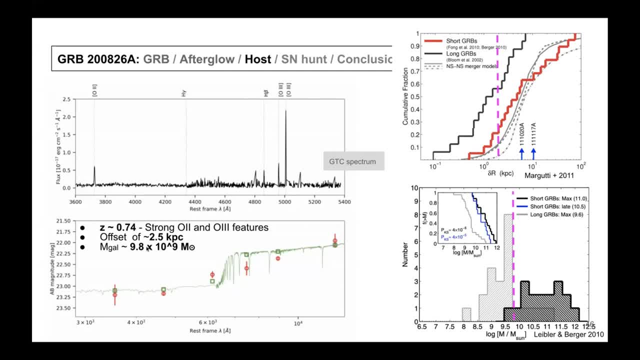 We can get the redshift, We can calculate how far from the center of the galaxy was this short GRV. So you have here, just next to my face. I guess that the long GRVs occur much closer to the center than short GRVs. 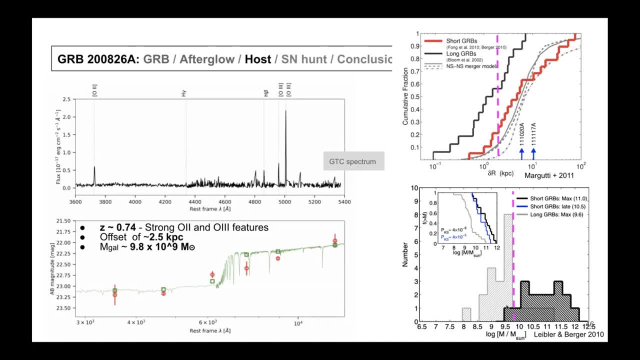 But this one was right in the middle. Usually the galaxies here, the plot on the bottom right. usually the galaxies are also more massive for short GRVs, But then you have here an overlap. This is the long GRV in gray. 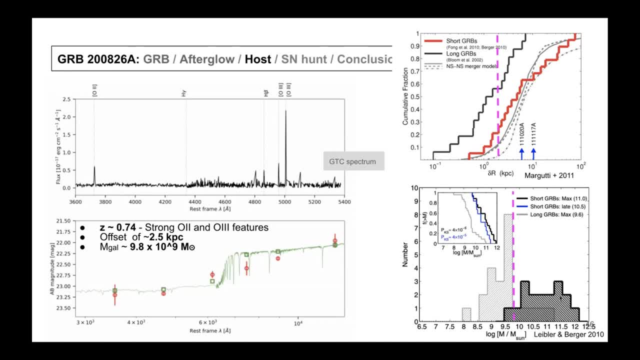 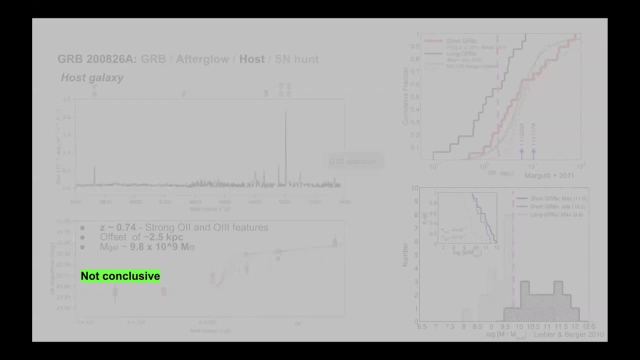 And then you have the short GRV in black And then exactly where they overlap is where our galaxy falls. So again, from this analysis it's basically not conclusive. We cannot say it's a collapsing massive star or it's a binary compact. 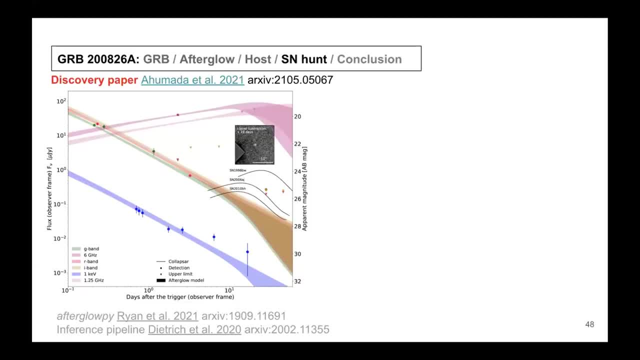 Then what can we do? We know that If it's a compact binary, it will produce a kilonova, But if it's a collapsing neutron star, it will produce a supernova. So you have here the light curve, You have the CTF data points. 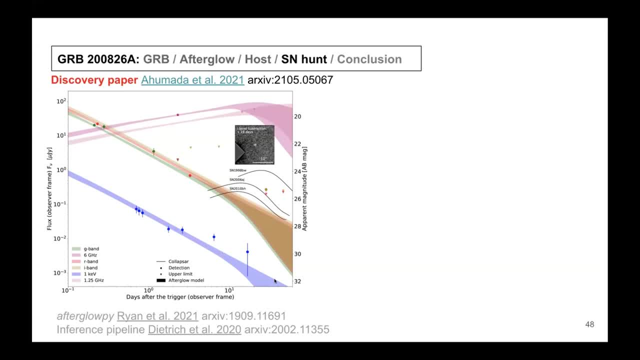 This is some radio here. This is the x-rays here. We have two more data points here And we know that this is declining. If we see something that goes above and there's like a supernova bump, sorry, you would definitely be able to say OK. 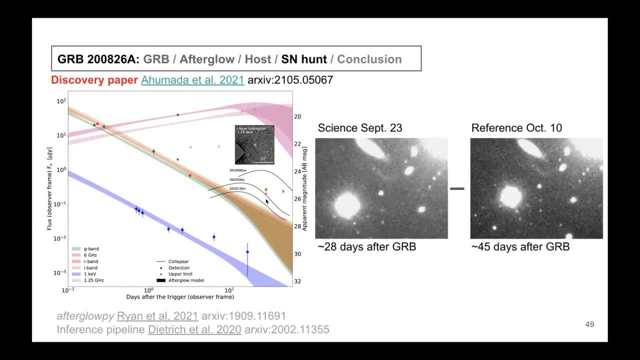 this is a compact binary. So what do we do? We took two different images with a very big telescope called the Gemini Observatory. You have here the science image that we took in September, then a reference image. We subtract those two And the difference shows this residual here. 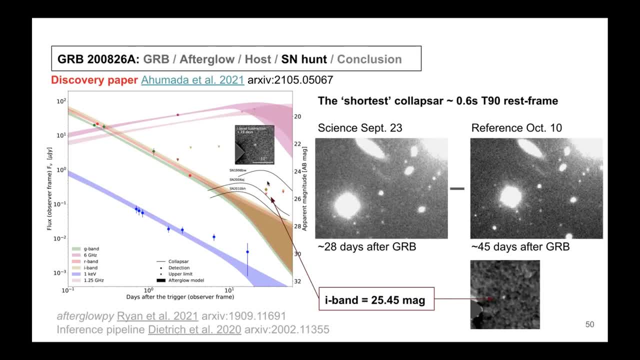 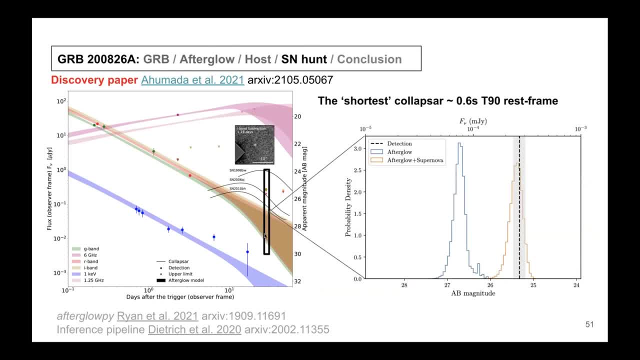 So what would we expect? So you have here the afterglow model. I'm slicing this here. This is the afterglow model, This is the detection. So you have that our models say that this thing, this detection, is too bright. 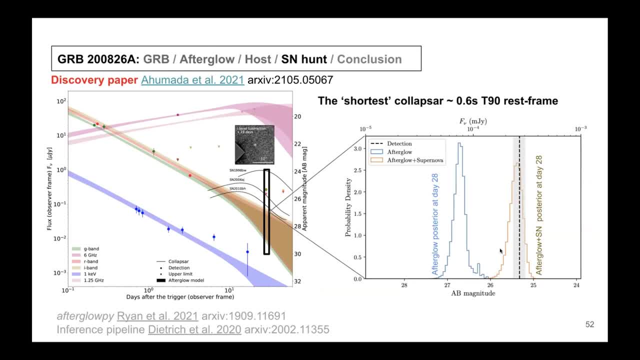 When we model the afterglow with a supernova component- it is one here in yellow- it falls right in the center. So with that we can say: OK, Yes, this is a supernova. that makes it the shortest collapse, because only in the rest frame lasted 4.6 seconds. 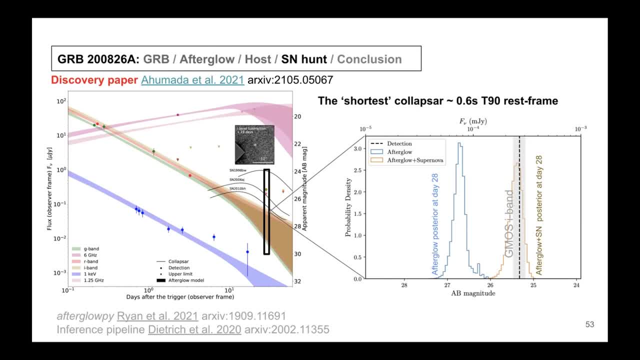 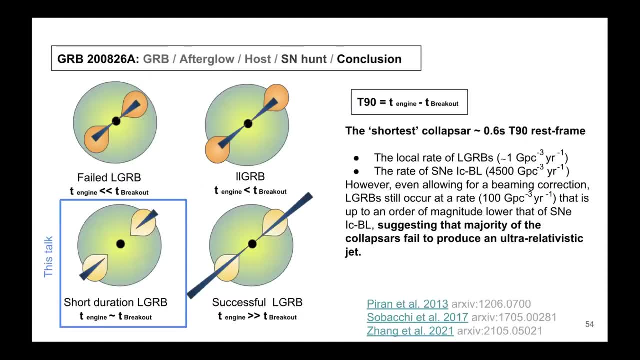 And that made it basically the shortest we've ever found. It also supports the scenario here in which you have an entire spectrum of sources that go from a star that collapses and fail to produce cherubis because, of course, the material was too thick. 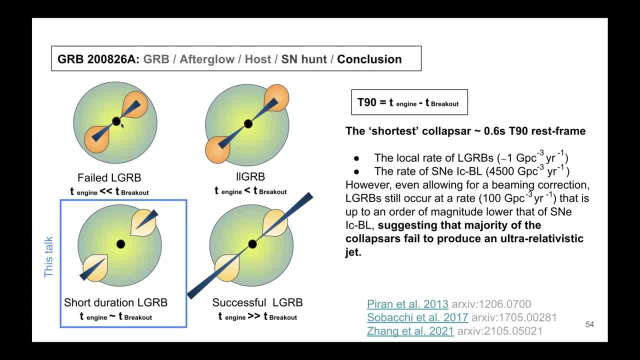 So it just didn't produce jets. But then they were shocked by the material around. Then you have low luminosity cherubis that are supposedly cherubis that died but did not made it through the surface, But the shock wave did. 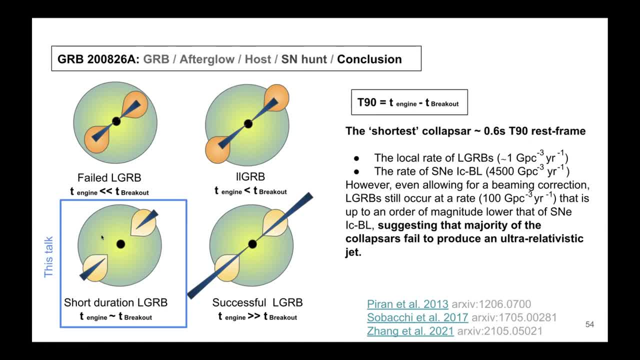 And then you have the one that I just presented, a short duration long cherubi, which is a cherubi that just made it. So you have here- the blue part is the cherubi- And then you have the successful long cherubi, which is the one. 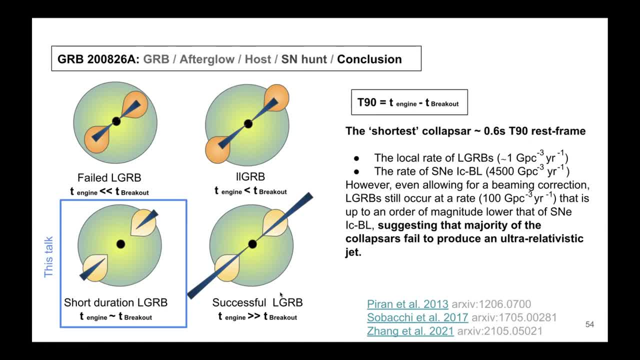 that is powering the jet constantly, And the amount of power that is injected is much larger than the one that you need to break through the surface. So you have this game, basically, of the duration between how much the engine is producing versus how much it will take you to go through the material. 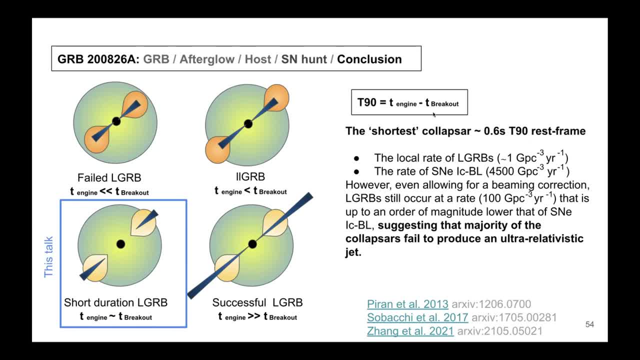 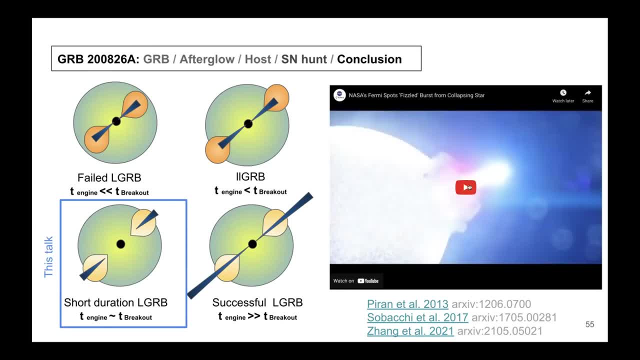 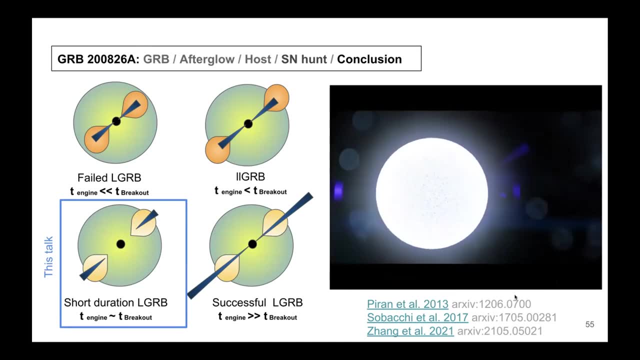 This work supports basically the claim that most of these collapsers fail to produce jets. I'm just going to show this one, Cherubi 20826.. Oops, And go and get some questions. So this is what we thought it happened. 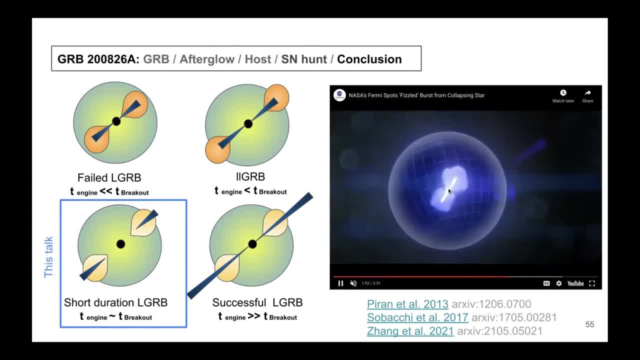 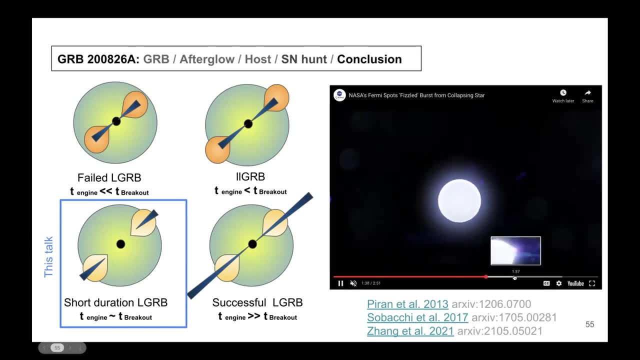 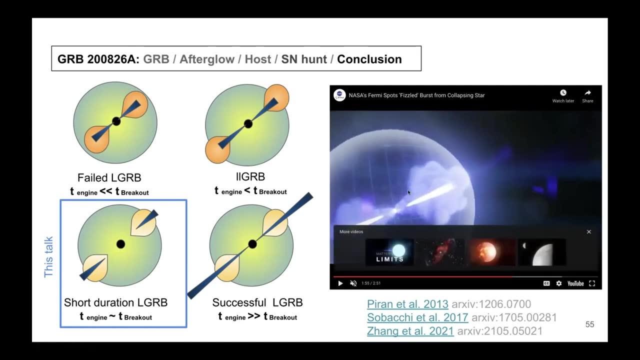 You have a massive star. It collapsed. It produced the jets And they were going around And then just going to stop that there. But what did I do? So if the jet dies here, you would see something like this scenario here. 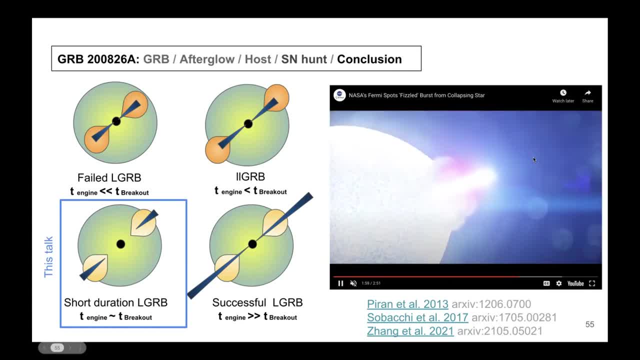 But it made it And then it's like boom, you have a cherubi, And then you have the jets, And then you have the afterglow, And then you have the supernova. But this is what we think happened. 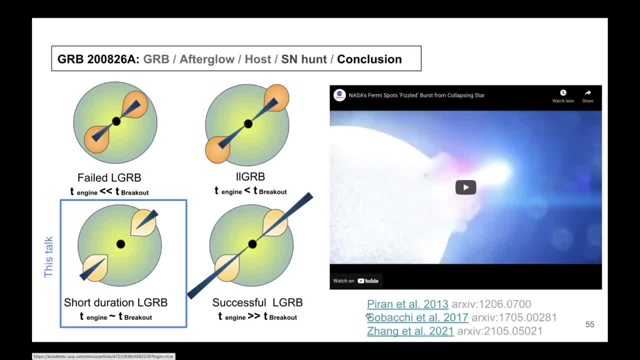 So So I'm just going to stop here and take questions. Really nice, Tomas. Are there questions from the room? OK, question from the room. I'm not able to see what was that envelope that was here. What is this envelope, Tomas? 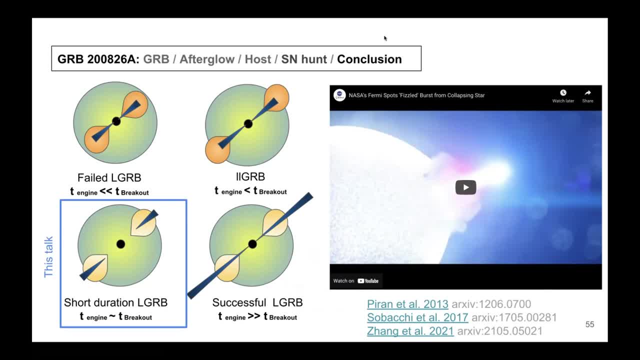 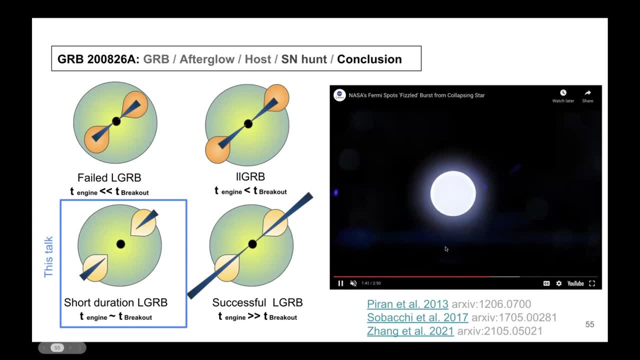 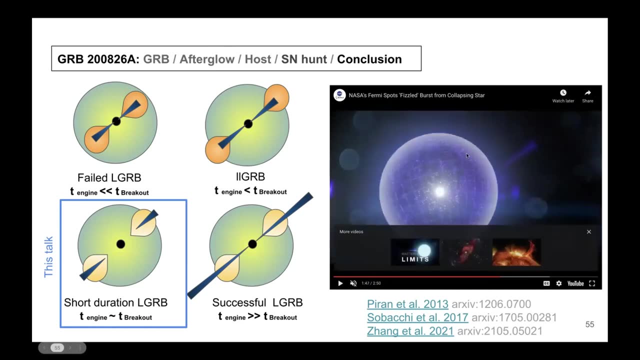 Say it again. I couldn't really hear. But what is this? What is the envelope? I guess you can see mine. Oh yeah, So the envelope is just the material of the star. Remember that the star has layers, And so I'm just going to here. 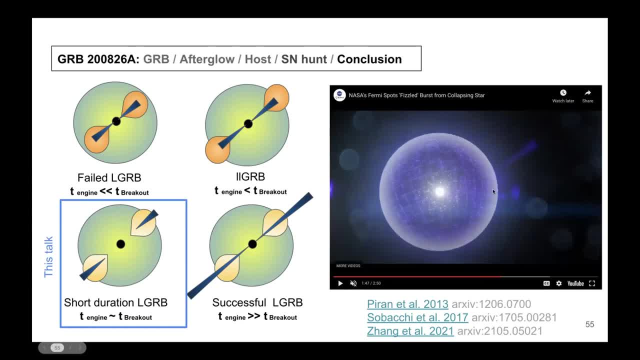 So you have this star And I guess the question is: what is this envelope? This envelope is actually the star. This is just happening in the very center of the star, where the material is collapsing, And it takes also a moment. OK, 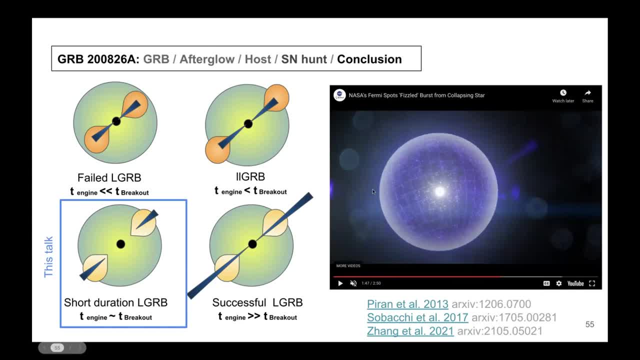 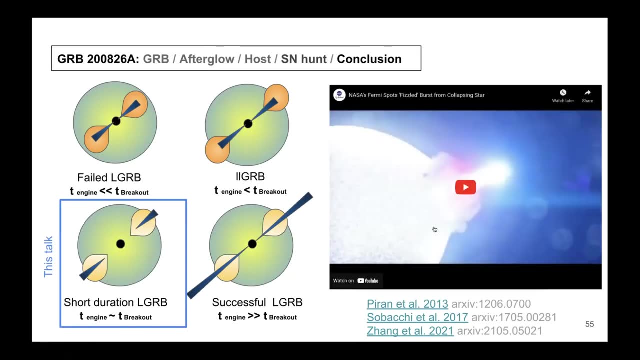 OK For the information to propagate. So the outer layers of the star do not really know that this is happening until they are swallowed by the or either pushed or swallowed by the material that is inside. Oops, I hope that helps. Any more questions from the room? 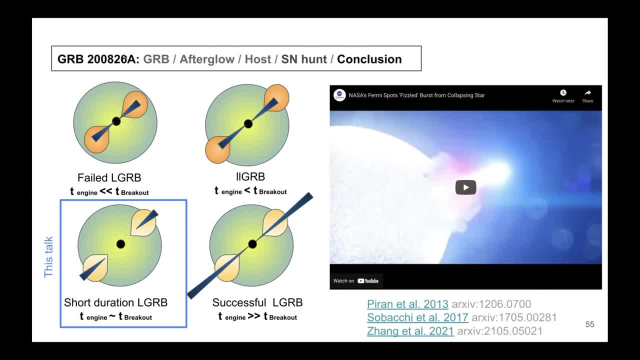 Yep, Would you please talk a little bit about what goes into calculating the breakouts? I guess I'm trying to understand What kind of physical situation would arise to get the kind of it seems like a perfect storm, almost Like is the star on the smaller end of the massive star? 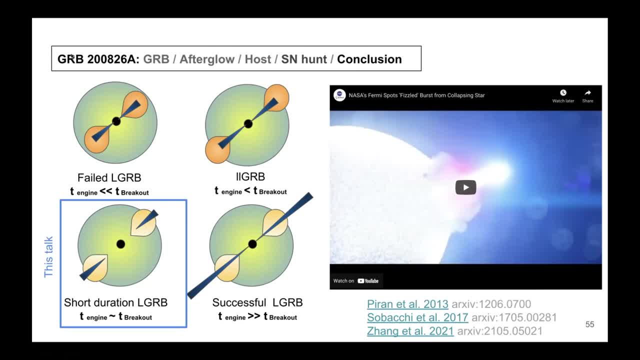 spectrum or Well, what does it go into calculating the T? You said breakout, So it basically is the size of the star, But it also depends on how bind it is OK, And also the composition. Different elements have different cross sections. 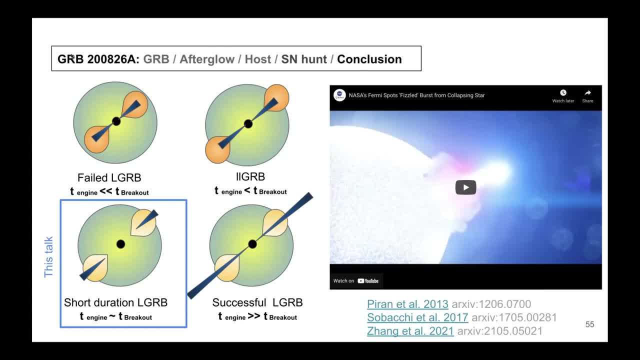 to neutrino radiation and stuff like that. So it also depends on the composition, the density. So you would expect that a smaller star. when you have this explosion in the center, it would be easier to get rid of everything because you have 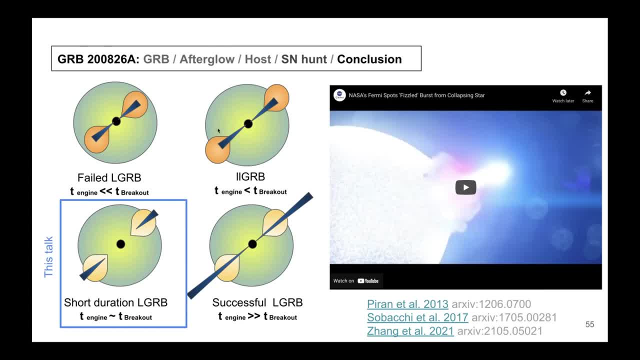 OK, You have less material, So probably it wouldn't really produce this long GRB, because if you push everything away then you'd have nothing to treat. So you have this sort of balance, because sometimes you don't really have to break out, because you